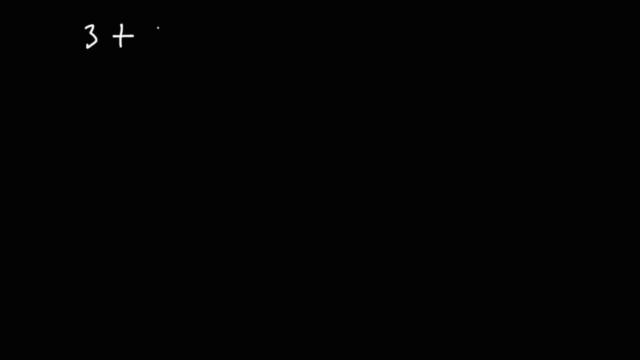 ahead and begin. So let's start with addition. What is three plus four? Now, when adding small numbers, a quick and simple way to find the answer is to use a number line. So here's zero. Positive numbers are on the right side, negative numbers on the left side. So first let's find the 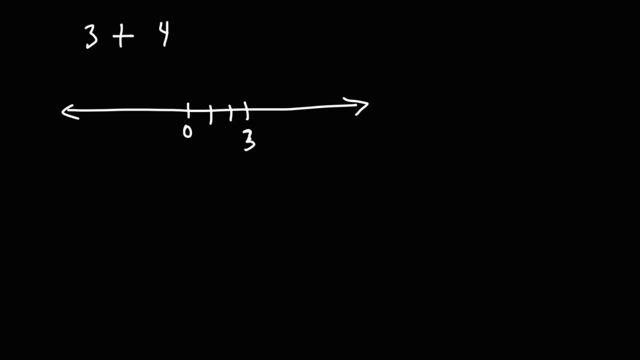 first number, which is three. Now, what you need to know is that when you're adding, move to the right of the number line. When you're subtracting, move to the left. So we're adding four to three. Thus, we need to move four units to the right. 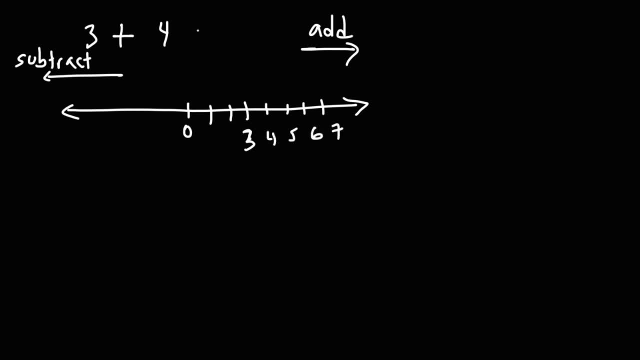 So this is four, Five, six, seven. Thus three plus four is seven. So let's try some more examples. Let's say we wish to add five and four, So let's start with the first number, five. Five is somewhere to the right of 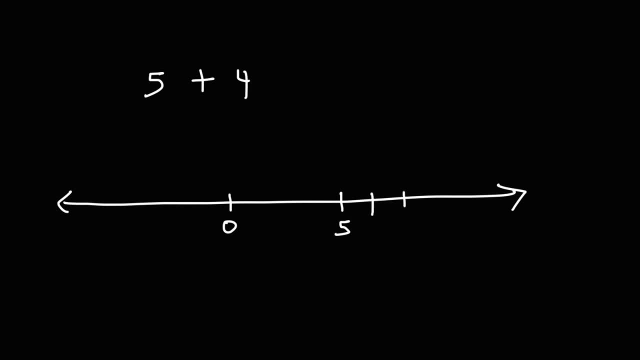 zero And then add four to five: One, two, three, four. So this is six, seven, eight, nine. Five plus four is nine. Now let's try some different examples. Let's say if we wish to add a negative number to a positive. 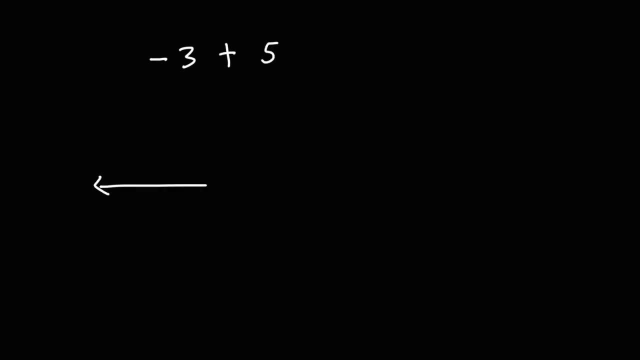 number Negative three plus five. What's the answer for that? So negative three is somewhere to the left of zero, So we're going to add five to it. One, two, this would be three, and then four, five. So this is. this ends at two. Negative three plus five is two. You can also reverse. 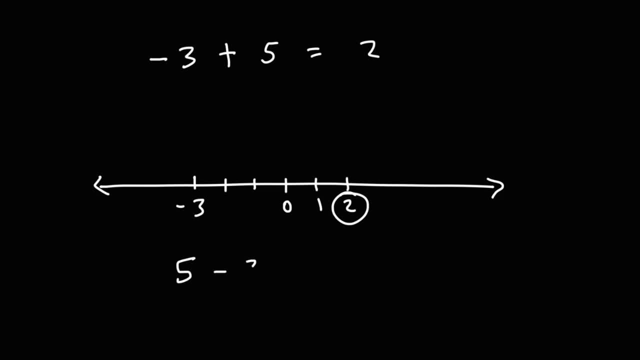 the numbers Negative. three plus five is the same as five minus three, which is also two. If you were to start at five and subtract it by three, that is, go three units to the left. this would be one, two and then three, which will take you to two as well. 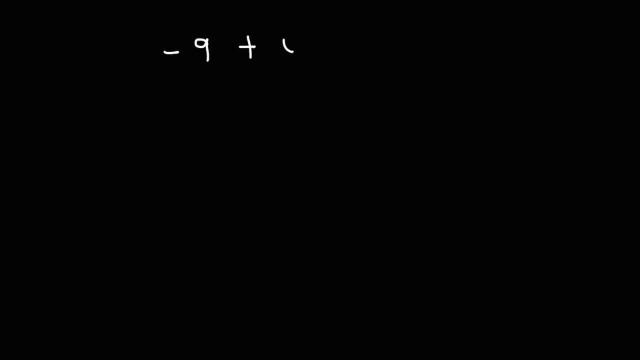 Now what about this example? What is negative nine plus four? Go ahead and try that. So negative nine is somewhere to the left of zero And we're adding four to negative nine, So we're going to travel four units to the right One. 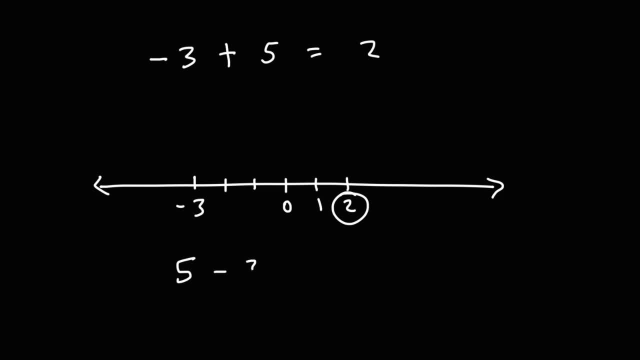 Negative. 3 plus 5 is the same as 5 minus 3. Which is also 2.. If you were to start at 5 and subtract it by 3. That is, go 3 units to the left, This would be 1,, 2, and then 3.. 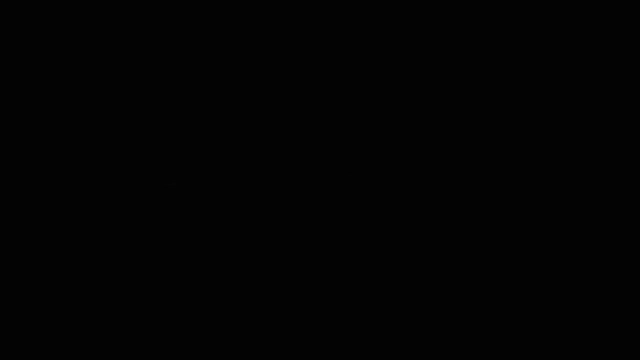 Which will take you to 2 as well. Now, what about this example? What is negative 9 plus 4?? Go ahead and try that. So negative 9 is somewhere to the left of 0. And we're adding 4 to negative 9.. 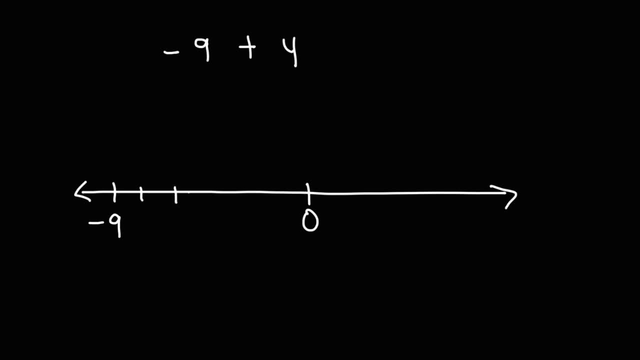 So we're going to travel 4 units to the right: 1,, 2,, 3,, 4.. So this is negative 8, negative 7, negative 6, and negative 5.. So negative 9 plus 4 is equal to negative 5.. 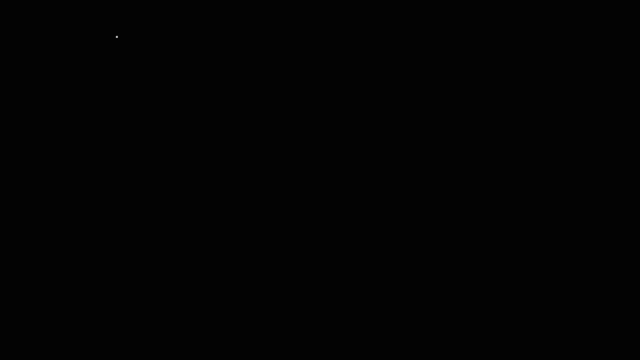 Now what about 4 minus 7 and also 5 minus 3?? So keep in mind when you're subtracting, move to the left. So let's start with 5.. Let's say this is 0 and 5 is over here. 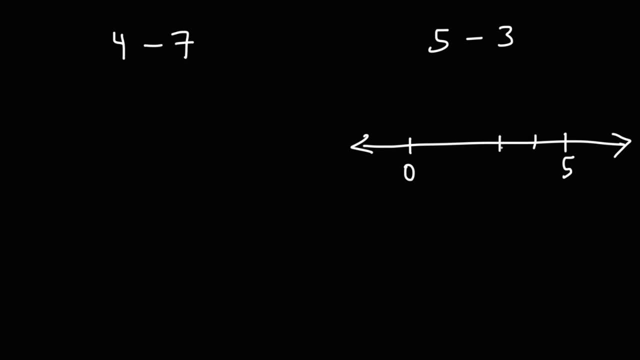 We need to move 3 units to the left: 1, 2, 3.. So 5 minus 3 is 2.. And then for 4 minus 7.. 4 is to the right of 0. So we're going to go 7 units to the left. 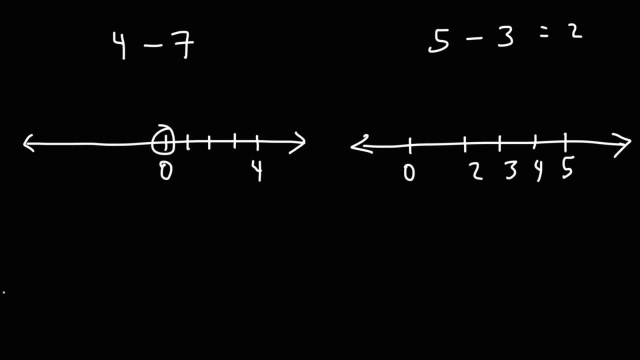 1, 2, 3. This is 4.. And then 5,, 6,, 7. This is negative 1,, negative 2, and negative 3.. So 4 minus 7 is negative 3.. 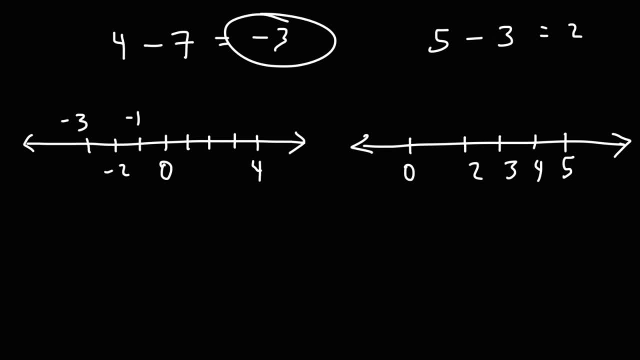 Drawing a number line really helps you in terms of when you need to add or subtract small numbers. Try this one: Negative 3 minus 5.. So I'm going to put the 0 here. Negative 3 is to the left of 0. 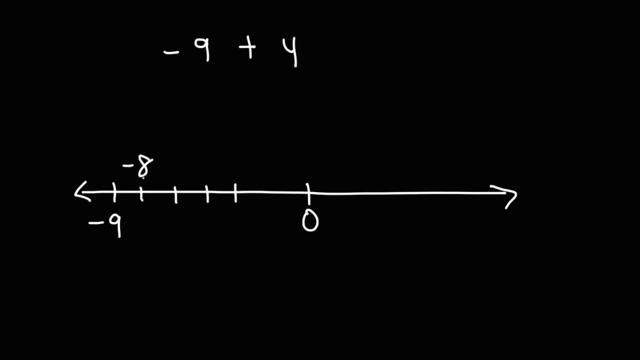 two, three, four. So this is negative eight. negative seven negative six. negative five. So negative nine plus four is equal to negative five. Now what about four minus seven? and also five minus three. So keep in mind when you're. 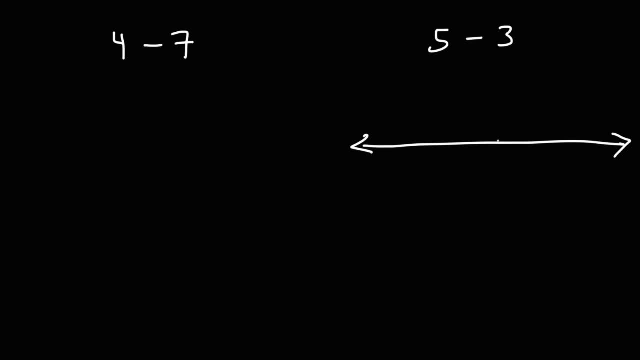 subtracting move to the left. So let's start with five. Let's say this is zero and five is over here. We need to move three units to the left: One, two, three. So five minus three is two, And then for four minus seven. 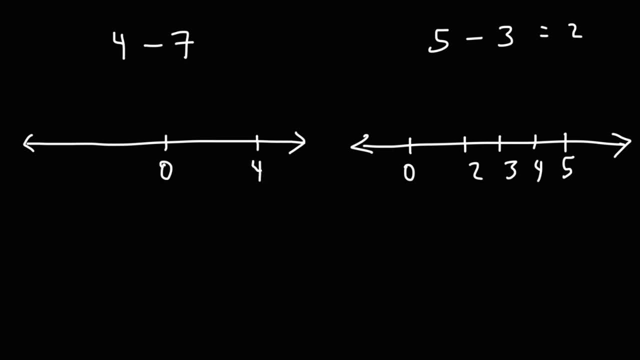 four is to the right of zero. So we're going to go seven units to the left: One, two, three, this is four, And then five, six, seven. This is negative, one negative two negative three. So four minus seven is negative three. 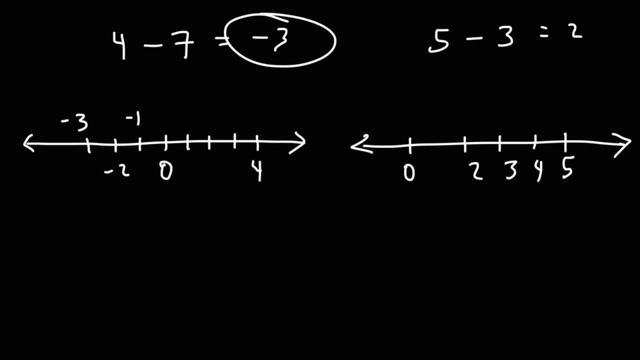 This drawing a number line really helps you in terms of when you need to add or subtract small numbers. Try this: one negative three minus five, So I'm going to put the zero here. Negative three is to the left of zero and we're subtracting it by five. 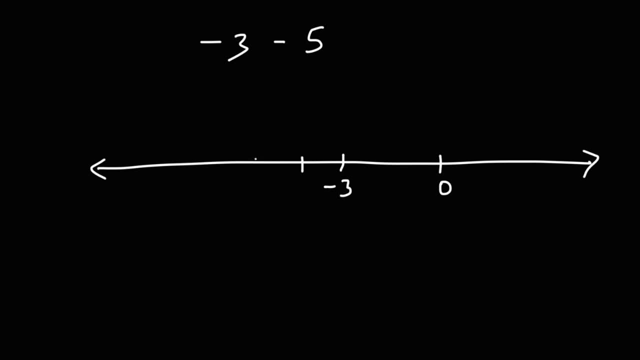 So we have to go five units to the left: One, two, three, four, five. So that's negative four, negative five, negative six, negative seven, negative eight. Thus negative three minus five is equal to negative eight. Now let's try some harder examples. What is six minus negative three? 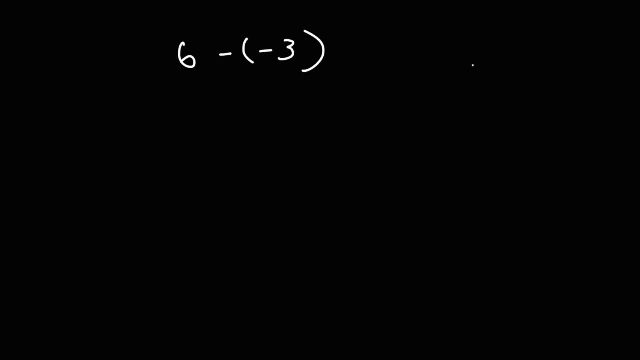 If you were to see that on the math test, what would you do? Whenever you have two negative signs next to each other, you're going to subtract five. So you're going to subtract five. So you're going to subtract five. If you were to see that on the math test, what would you do Whenever you have two negative signs next to each other? 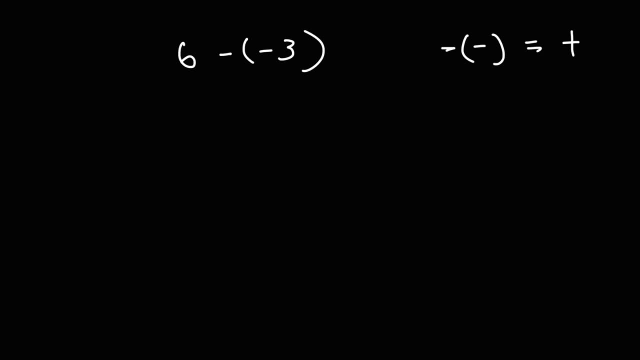 it's equal to a positive sign. A negative times a negative is equal to a positive number. So six minus negative three can be converted into six plus three. You could change these two negative signs to a positive sign And six plus three if you start with six and then move three units to. 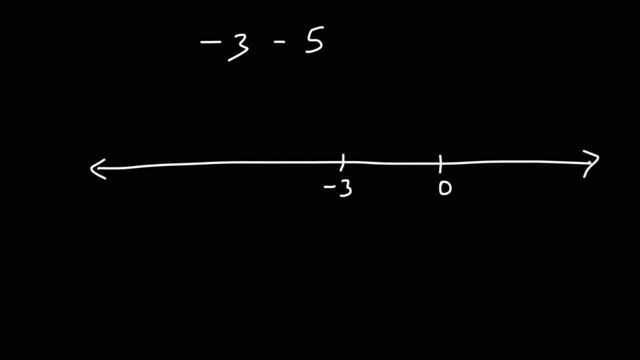 And we're subtracting it by 5.. So we have to go 5 units to the left: 1, 2, 3, 4, 5.. So that's negative 4, negative 5, negative 6, negative 7, negative 8.. 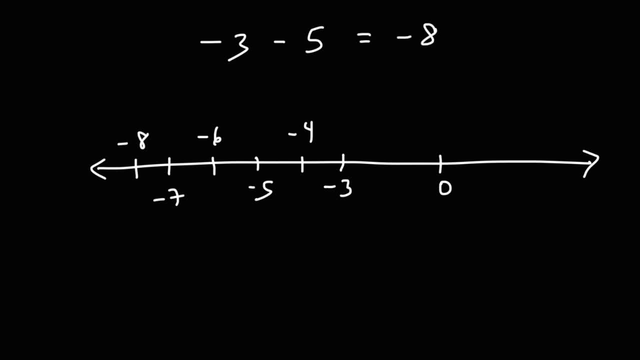 Thus negative 3 minus 5 is equal to negative 8.. Now let's try some harder examples. What is 6 minus negative 3?? If you were to see that on the math test, what would you do Whenever you have two negative signs next to each other? 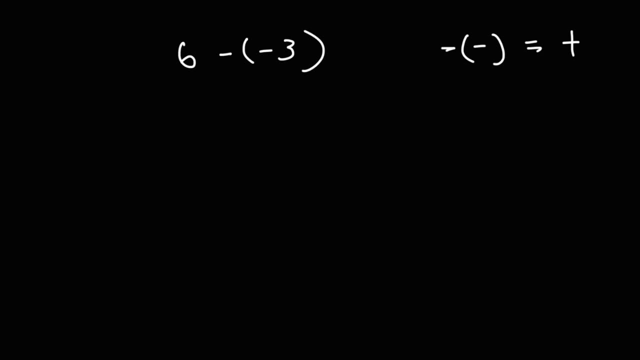 it's equal to a positive sign. A negative times a negative is equal to a positive number. So 6 minus negative 3 can be converted into 6 plus 3.. You could change these two negative signs to a positive sign And 6 plus 3, if you start with 6 and then move 3 units to the right. 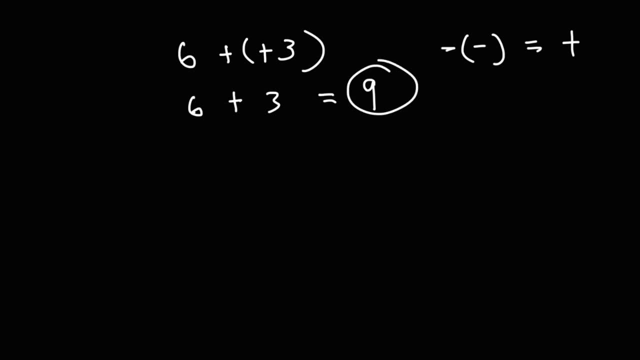 this will equal 9.. Now what about an example that looks like this: Negative 7 minus negative 3.. If you see that we could do the same thing, We could change the two negative signs that are next to each other with a positive sign. 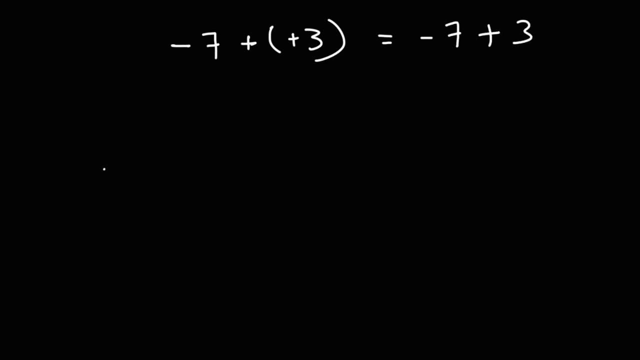 So this is negative 7 plus 3.. And then at that point we could use the number line to get the answer. So, starting from negative 7,, we're going to travel 3 units to the right: 1,, 2,, 3.. 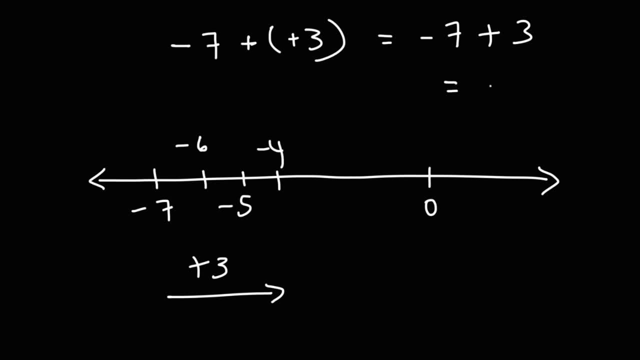 Negative 6, negative 5, negative 4.. So negative 7 plus 3,, which is the same as negative 7 minus negative 3. That is equal to negative 4.. So that's how you can form addition and subtraction with simple integers. 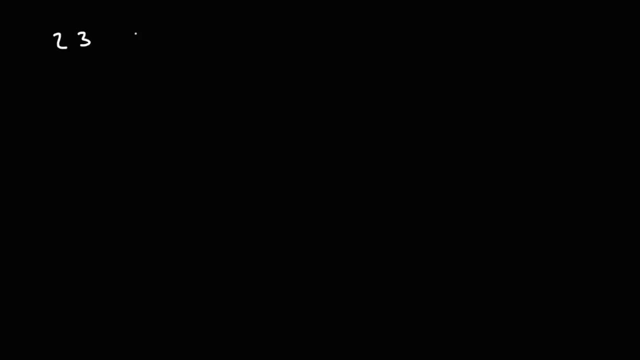 Now what about adding larger numbers? Let's say 23 plus 45. How can we do this? Well, in school you've seen problems like this, where you can just align them up together and then add. So first you would add 5 and 3, which is 8.. 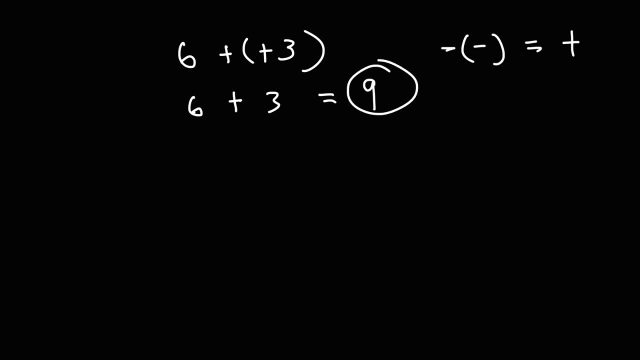 the right, this will equal nine. Now what about an example that looks like this: Negative seven minus negative three. If you see that we could do the same thing, We could change the two negative signs that are next to each other with a positive sign. So this is negative seven plus three, And 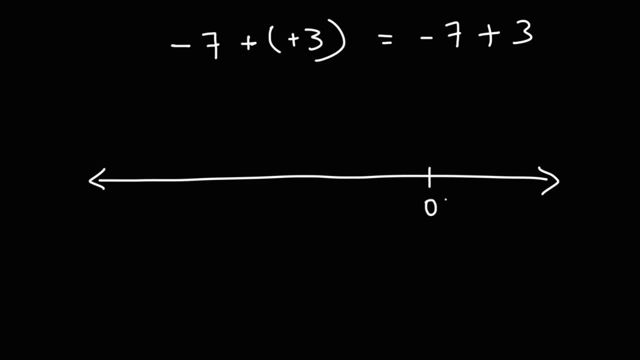 then at that point we could use a number line to get the answer. So, starting from negative seven, we're going to travel three units to the right: One, two, three Negative six, negative five, negative four. So negative seven plus three. 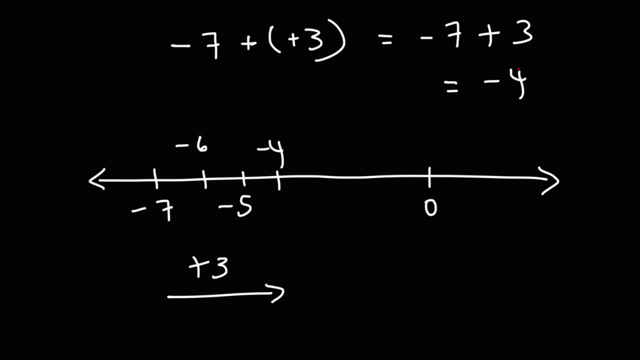 which is the same as negative seven minus negative three, That is equal to negative four. So that's how you can form addition and subtraction with simple integers. Now what about adding larger numbers? Let's say 23 plus 45. How can we do this? Well, in school. 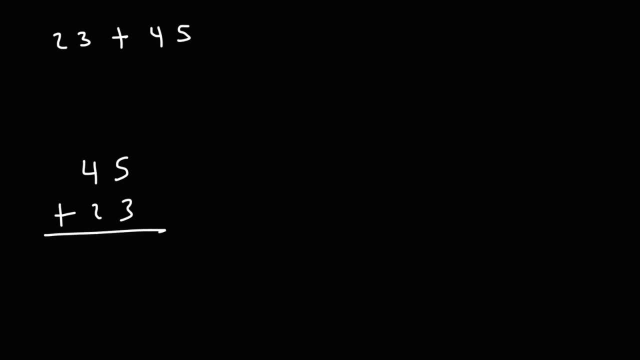 you've seen problems like this, where you can just align them up together and then add. So first you would add five and three, Which is eight, And then four and two, which is six, And that's it for that one. Now, what about this one? 35 plus 49.. Well, we could follow the same process. 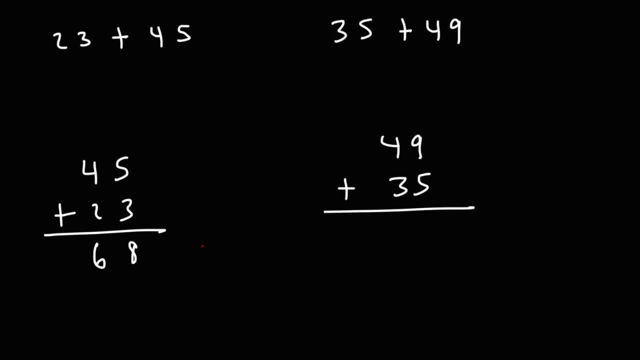 but this one's going to be a little different. So first we would add nine and five. Nine plus five is 14.. Now we won't write 14 on the bottom, We'll write four and then carry over the one. 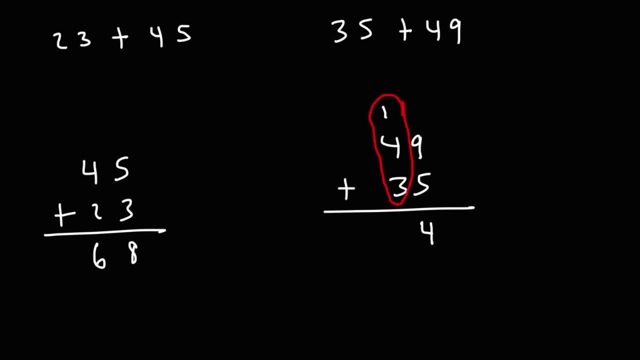 Next we'll move to the next column and then add one plus four plus three, which is eight. So 49 plus 35 is 84.. Try this. Add 236 plus 185.. Feel free to pause the video and work on that example. 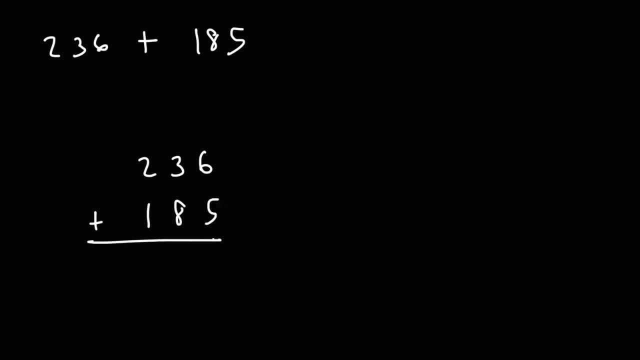 So we could use the same process here. Six plus five is 11.. Write the one, carry over the other one, And then we're going to add three. add this column of numbers: 1 plus 3 is 4.. 4 plus 8 is 12.. Write the 2, carry over the 1,. 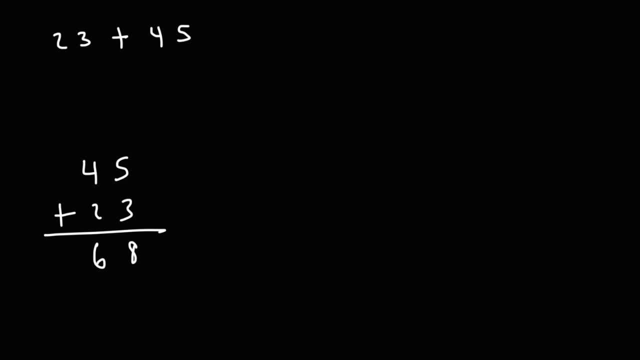 And then 4 and 2, which is 6.. And that's it for that one. Now, what about this one? 35 plus 49.. Well, we could follow the same process, but this one's going to be a little different. 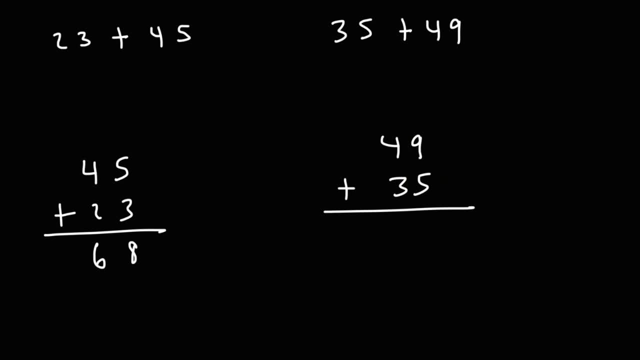 So first we would add 9 and 5.. 9 plus 5 is 14.. Now we won't write 14 on the bottom, We'll write 4 and then carry over the 1.. Next we'll move to the next column and then add 1 plus 4 plus 3, which is 8.. 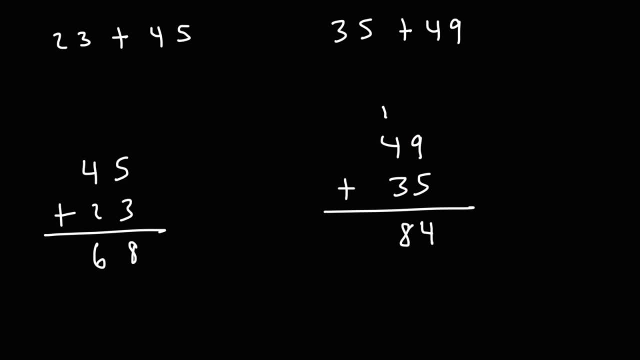 So 49 plus 35 is 84.. Try this. Add 236 plus 185.. Feel free to pause the video and work on that example So we could use the same process here. 6 plus 5 is 11.. Write the 1, carry over the other 1.. 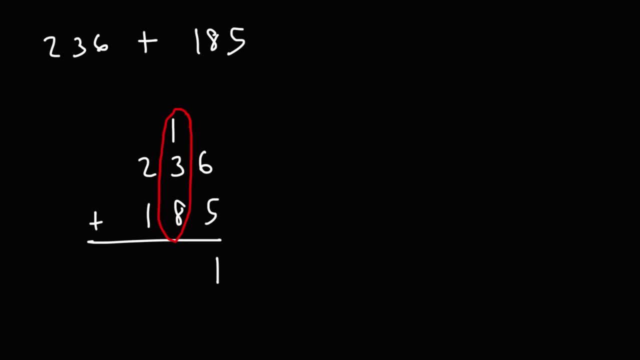 And then we're going to add this column of numbers: 1 plus 3 is 4.. 4 plus 8 is 12.. Write the 2, carry over the 1. And then 1 plus 2 plus 1 is 4.. 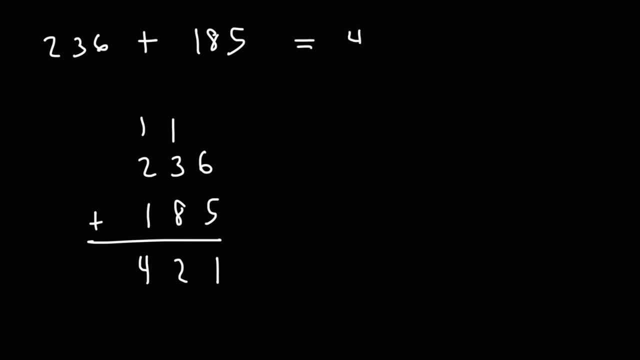 So 236 plus 185 is 421.. And when working out these problems it's good to check your work to make sure you have it right. So you can take a calculator and just type in 236 plus 185 and just make sure that you have the right answer. 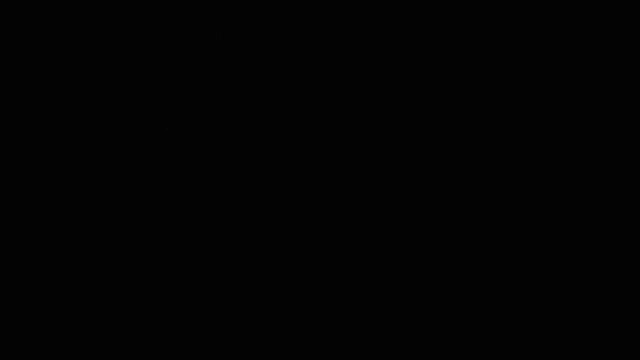 So that's how you could do addition with larger numbers. Now let's consider subtracting large numbers. Try these three examples: 96 minus 63., 73 minus 45. And also 136 minus 58.. So let's start with the first one. 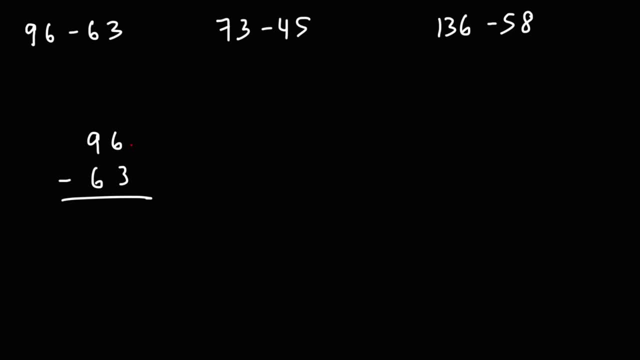 96 minus 63.. So what you're going to do is you're going to focus on each column and subtract the large number by the small number. 6 minus 3 is 3.. I mean, subtract the top number by the number on the bottom. 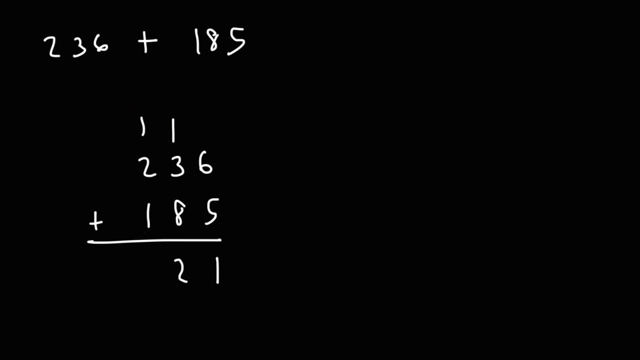 and then 1 plus 2 plus 1 is 4.. So 236 plus 185 is 421.. And when working out these problems it's good to check your work to make sure you have it right. So you can take a calculator and 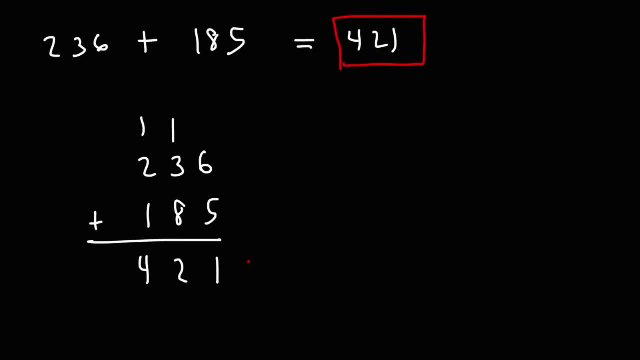 type in 236 plus 185 and just make sure that you have the right answer. So that's how you could do addition with larger numbers. Now let's consider subtracting large numbers. Try these three examples: 96 minus 63,, 73 minus 45, and also 136 minus 58.. So let's start with the first one. 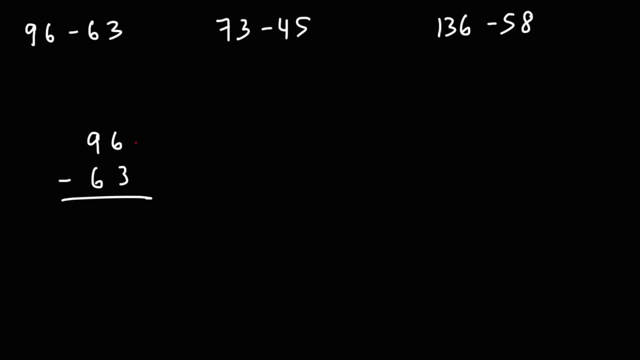 96 minus 63.. So where are you going to type in the numbers? going to do is you're going to focus on each column and subtract the large number by the small number. 6 minus 3 is 3.. I mean subtract the top number by the number on the bottom, because 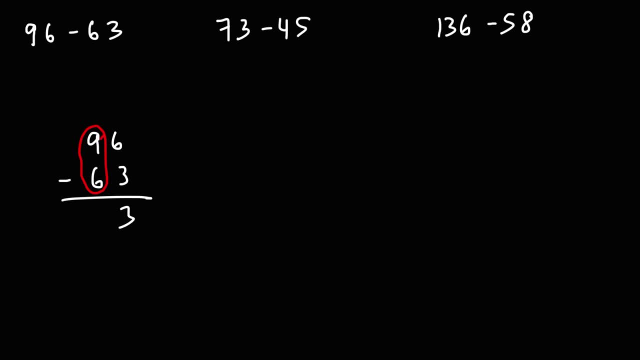 sometimes the top number is not always the large number. 9 minus 6 is 3.. So the answer is 33 for the first example. Now for the second example. this one is different, So we're going to take the top number subtracted by the bottom number. 3 minus 5 is a negative number, so we need 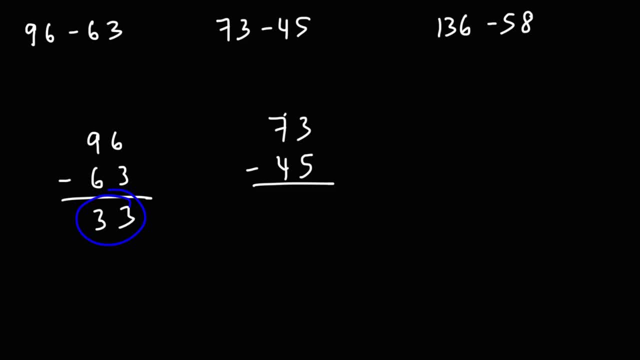 to do something different here. What we're going to do is borrow a 1 from the 7. So the 7 becomes a 6. The 3 becomes 13.. Now we can subtract 13 by 5, which is 8.. And then we can subtract 6 by 4. 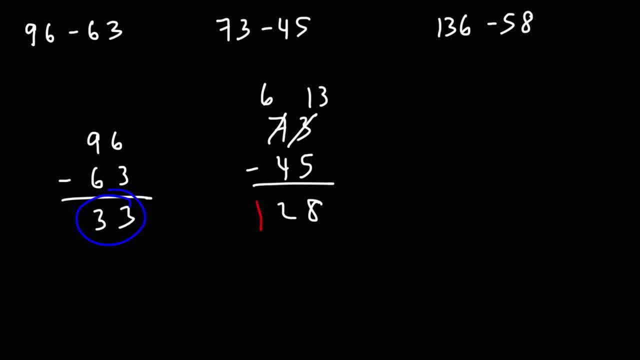 which is 2.. So we have the answer: 73 minus 45 is 28.. And you can compare the two. So we have the answer: 73 minus 45 is 28.. And you can compare the two. Let's confirm that with the calculator. Now let's move on to the next one: 136 minus 58.. So once. 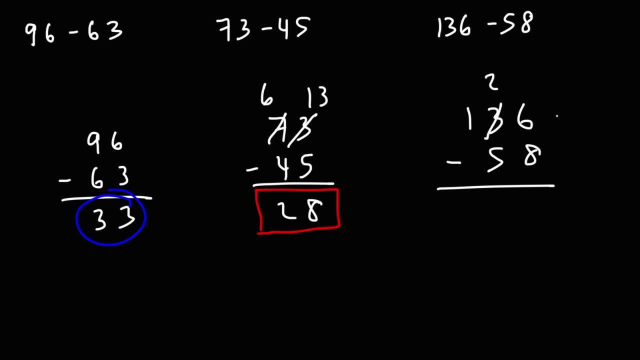 again, we need to borrow a 1 from the 3. This becomes a 2.. The reason for that is: 6 minus 8 is negative, so we need to borrow a 1.. Thus the 6 becomes a 16.. Now we can subtract 16 by 8, which 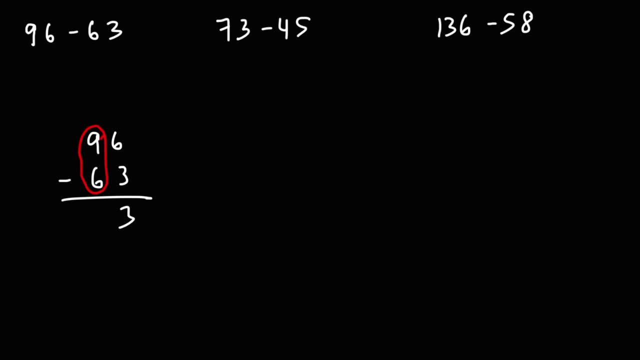 Because sometimes the top number is not always the large number. 9 minus 6 is 3.. So the answer is 33 for the first example. Now for the second example. this one is different. So we're going to take the top number and subtract it by the bottom number. 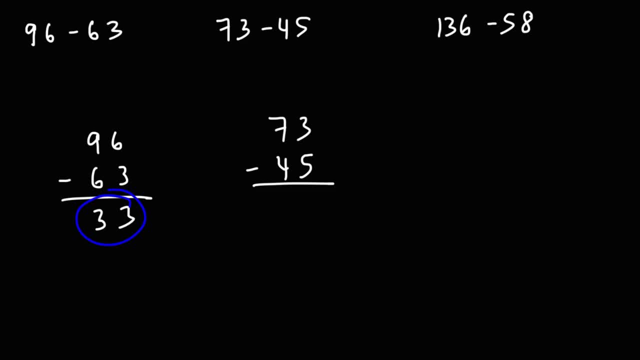 3 minus 5 is a negative number, so we need to do something different here. What we're going to do is borrow a 1 from the 7. So the 7 becomes a 6. The 3 becomes 13.. 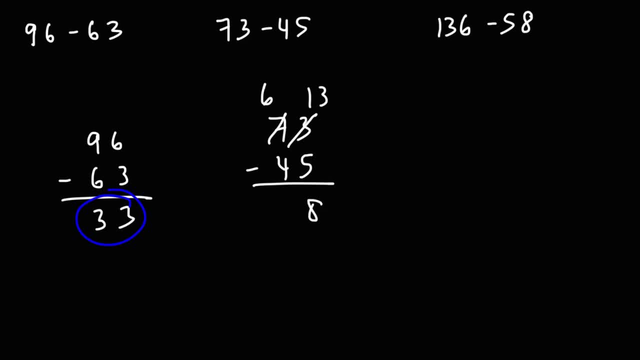 Now we can subtract 13 by 5,, which is 8.. And then we can subtract 6 by 4,, which is 2.. So we have the answer: 73 minus 45 is 28.. And you can confirm that with the calculator. 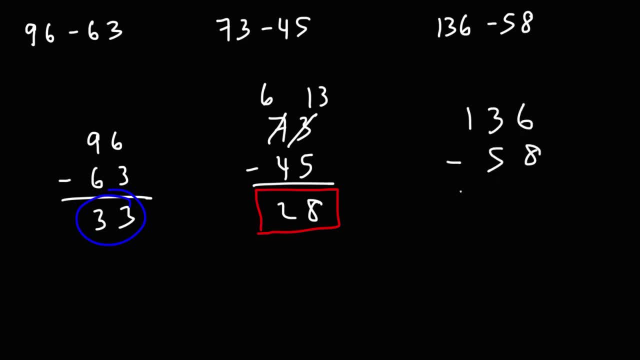 Now let's move on to the next one: 136 minus 58.. So once again, we need to borrow a 1 from the 3. This becomes a 2.. The reason for that is: 6 minus 8 is a negative, so we need to borrow a 1.. 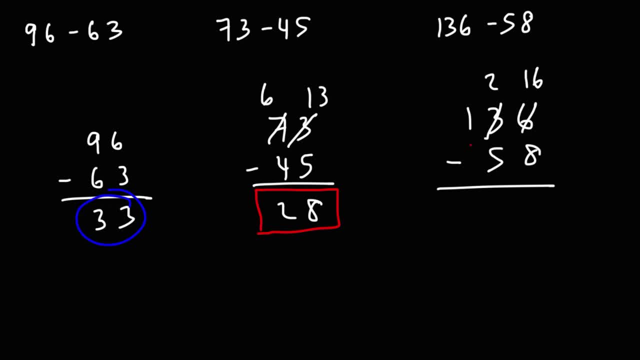 Thus the 6 becomes a 16.. Now we can subtract 16 by 8, which will give us 8. And we can't subtract 2 by 5, because that's going to give us a negative number. So we need to borrow a 1.. 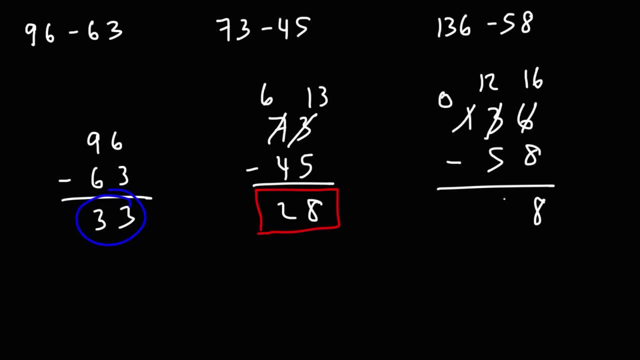 That becomes 0. This becomes 12.. 12 minus 5 is 7.. So 136 minus 58 is 78.. Thus, that's how you can subtract large numbers, And now you know how to borrow a 1 when needed. 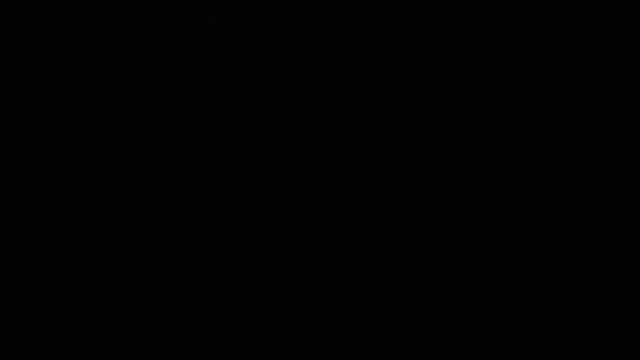 Now let's move on to the next topic of discussion, and that is multiplication. So let's say: if we want to multiply 4 by 3.. You can write it that way. This also means multiplication, That's 4 times 3.. 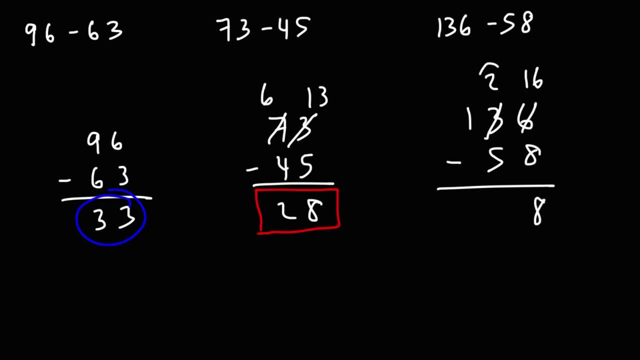 will give us 8. And we can't subtract 2 by 5 because that's going to give us a negative number. So we need to borrow a 1 from the 3. And we can't subtract 2 by 5, because that's going to give us: 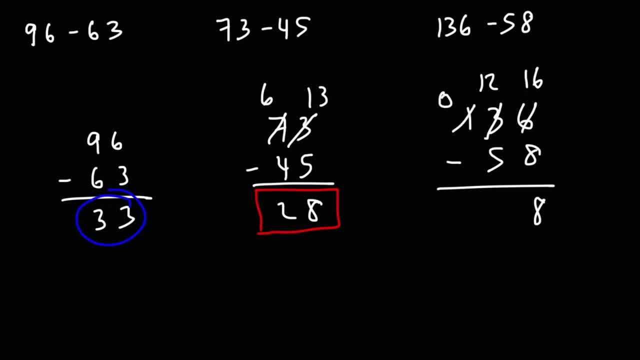 a negative number, So we need to borrow a 1. That becomes 0. This becomes 12.. 12 minus 5 is 7.. So 136 minus 58 is 78.. Thus, that's how you can subtract large numbers, And now you know how to. 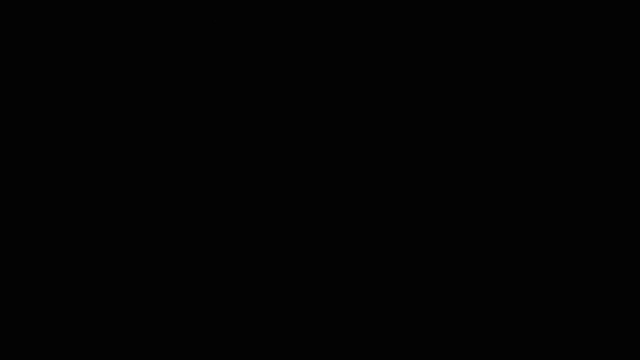 borrow a 1 when needed. Now let's move on to the next topic of discussion, and that is multiplication. So let's say, if we want to multiply 4 by 3. You can write it that way. This also means that we can: 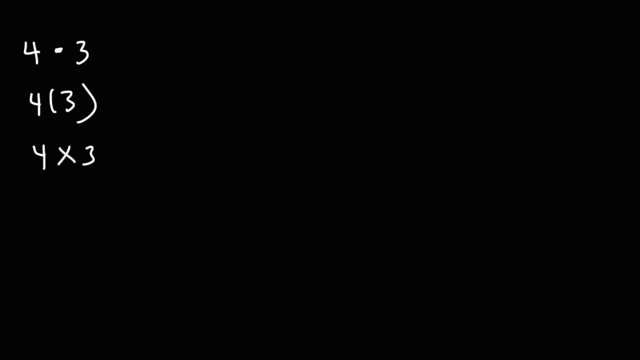 means multiplication, that's 4 times 3, or you could put an x in the middle. All of these are different ways to represent multiplication. But what is 4 times 3?? Multiplication is repeat addition. So 4 times 3 means that you're adding 4 three times. It also means that you're adding 3. 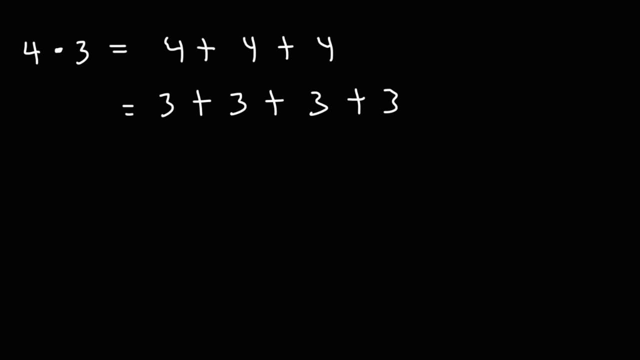 four times. You could view it both ways: 4 plus 4 is 8, and then 8 plus 4 is 12.. 3 plus 3, that's 6, and add in the other two threes on the right, that's 6.. 6 plus 6 is 12.. 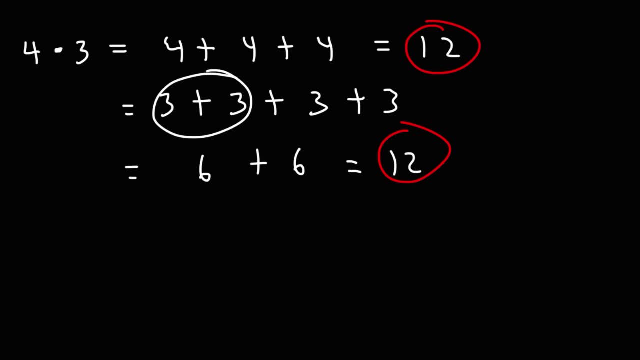 In both cases you get the same answer. So that's multiplication, repeat addition. Now let's say: if we want to multiply 7 times 3,, we're going to multiply 7 times 3, and then we're going to add 7 by 3.. Now you can add 7 three times, or you can add 3 seven times. It's easier adding 7. 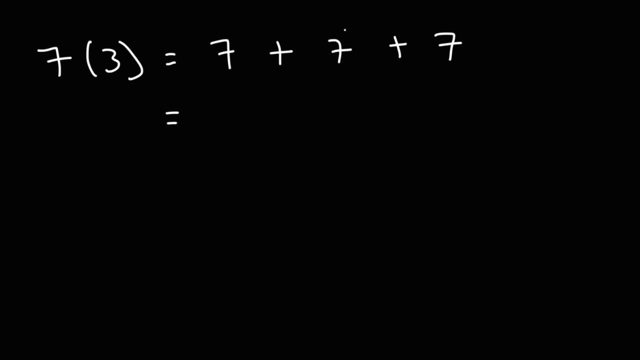 three times. so I'm going to go with that route. 7 plus 7 is 14,, and 14 plus 7 is 21.. And so that's 7 times 3.. So this method helps you to understand how multiplication works. It's simply repeat. 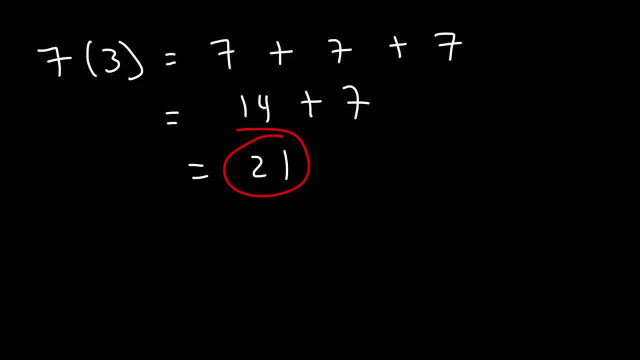 addition, But nevertheless, I recommend that you memorize. So it might be wise for you to go to Google Images, look up the multiplication table up to 12 times 12, and just memorize those values, because that's going to help you when multiplying. 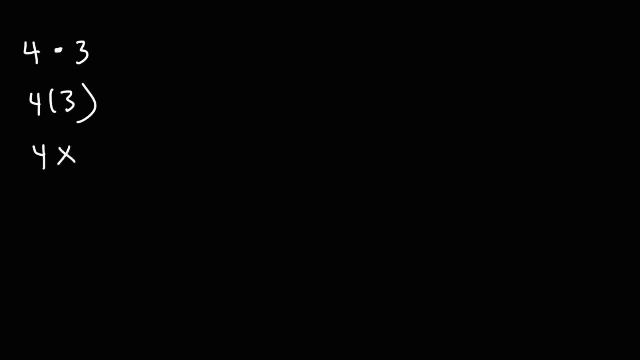 Or you can put an x in the middle. All of these are different ways to represent multiplication. But what is 4 times 3?? Multiplication is repeat addition. So 4 times 3 means that you're adding 4 three times. 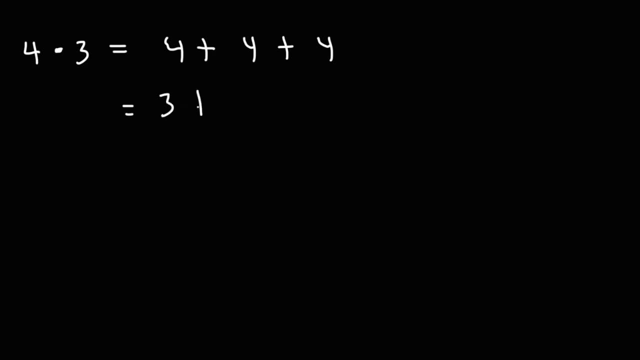 It also means that you're adding 3 four times. You could view it both ways: 4 plus 4 is 8.. And then 8 plus 4 is 12.. 3 plus 3, that's 6.. And add in the other two 3's on the right, that's 6.. 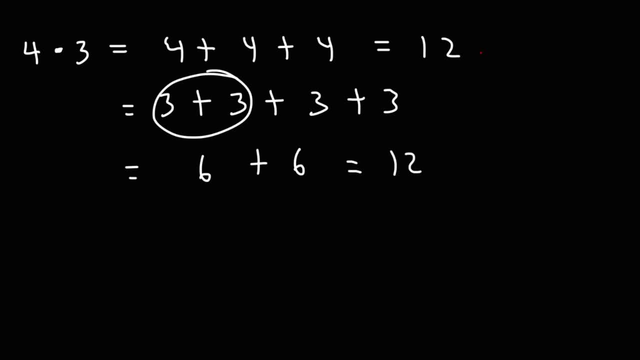 6 plus 6 is 12.. In both cases you get the same answer. So that's multiplication, Repeat addition. Now let's say if we want to multiply 7 by 3. Now you can add 7 three times. 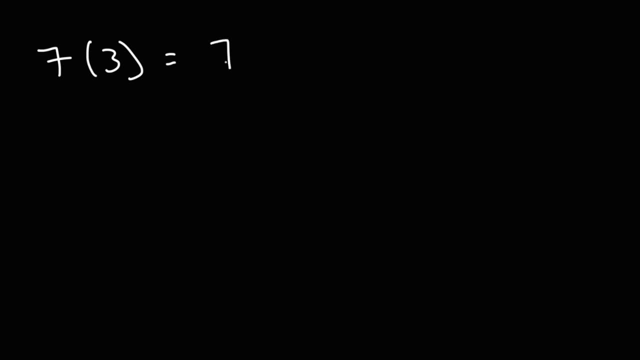 Or you can add 3.. 7 times. It's easier adding 7 three times, So I'm going to go with that route. 7 plus 7 is 14. And 14 plus 7 is 21. And so that's 7 times 3.. 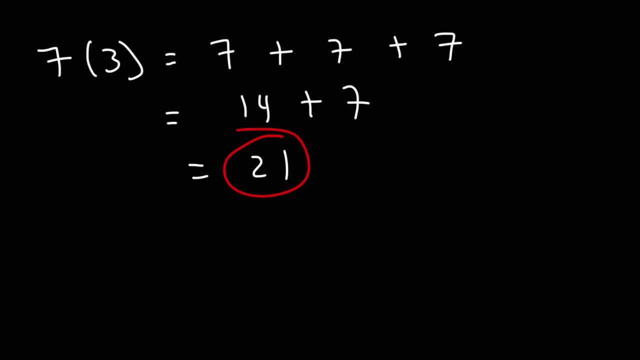 So this method helps you to understand how multiplication works. It's simply repeat addition, But nevertheless, I recommend that you memorize the multiplication table up to 12.. So it might be wise for you to go to Google Images, Look up the multiplication table up to 12 times 12.. 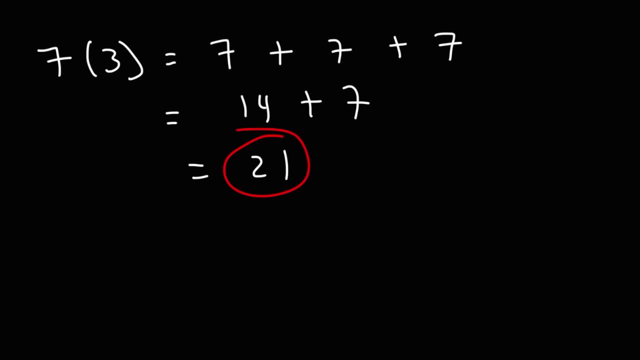 And just memorize those values, Because that's going to help you when multiplying other numbers, Such as 8 times 6. Or 9 times 5. Or 7 times 4.. It's good to memorize the answers for these. 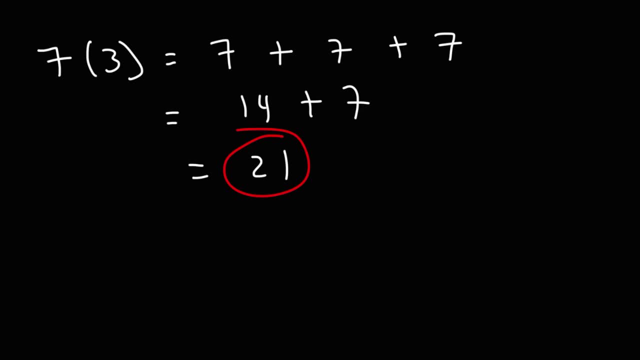 It'll make math a lot easier. But if you don't want to memorize it, you could do it the hard way, Which is writing it out. For instance, let's say, if you want to multiply 8 by 6. So the best thing to do is add 8 six times. 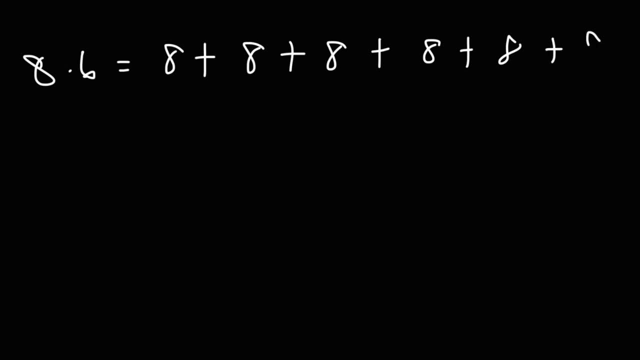 Instead of adding 6, 8 times. So 8 plus 8 is 16.. So this is 16 here, That's 16. And that's 16.. Now, 16 plus 16 is 32.. And 32 plus 16 is 48.. 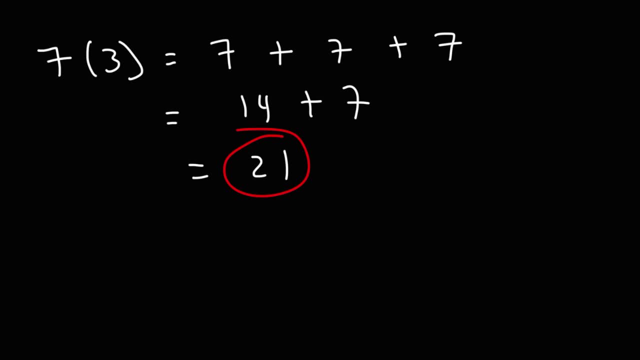 other numbers, such as 8 times 6, or 9 times 5, or 7 times 4.. It's good to memorize the answers for these. It'll make math a lot easier. But if you don't want to memorize it, 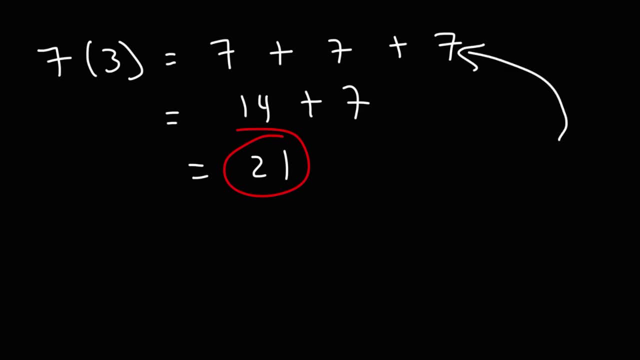 you could do it the hard way, which is writing it out. For instance, let's say, if you want to multiply 8 by 6.. So the best thing to do is add 8 six times instead of adding 6 eight times. 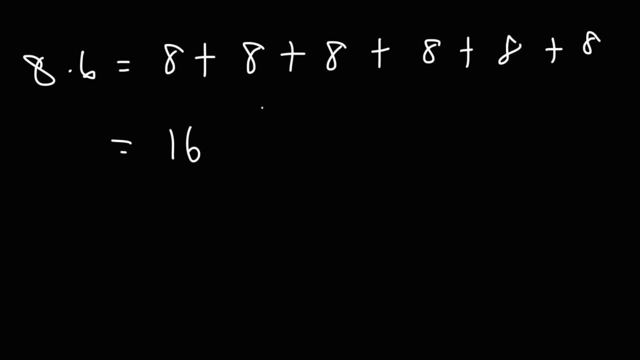 So 8 plus 8 is 16.. So this is 16 here, that's 16, and that's 16.. Now, 16 plus 16 is 32.. And 32 plus 16 is 48. So 8 times 6, which is the same as 6 times 8, that's 48. I definitely think. 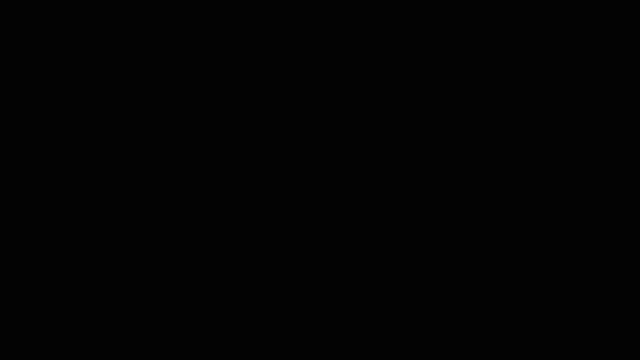 it's wise that you commit the multiplication table to memory, for those of you who really want to learn this. Now let's talk about multiplying large numbers. What is 16 times 7?? Well, one technique you could use is long multiplication. First, you can multiply 6 times. 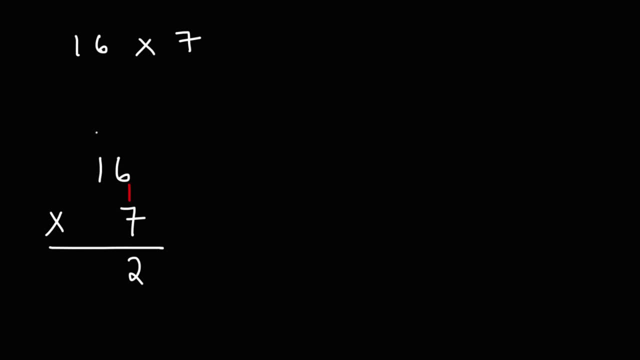 7,, which is 42. What you need to do is write the 2,, carry over the 4, and then multiply 7 times 1,, which is 7, and then add the 4.. 7 plus 4 is 11.. Thus, 16 times 4 is 112.. Another way in which 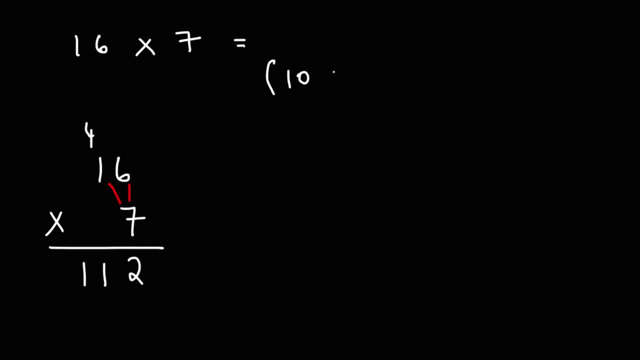 you could do this is you could break up 16 into two numbers. 10 plus 6 is 16. And then you could use the distributive property. 10 times 7 is 7. And then you could use the distributive property. 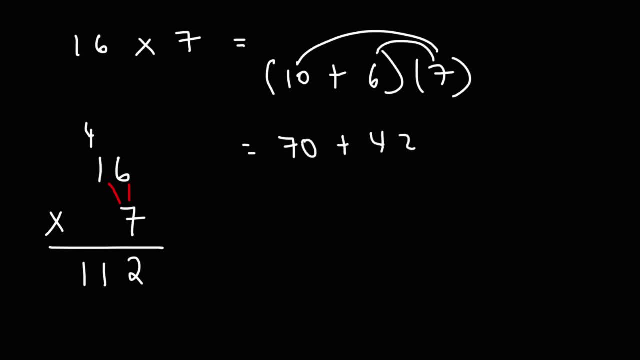 And 7 times 6 is 42. And so you're adding 70 and 42 together, which is 112.. So that's another way in which you can get the same answer. Now, what about 20 times 17?? What's the answer for that? 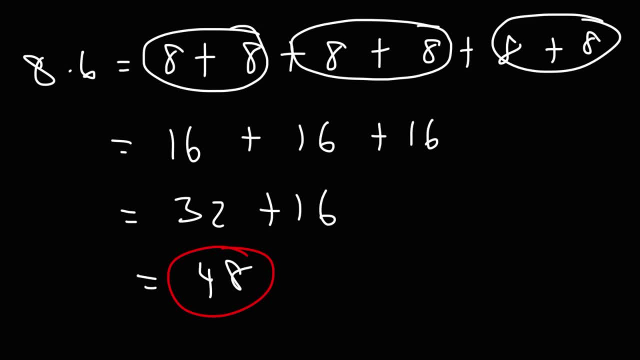 So 8 times 6, which is the same as 6 times 8.. That's 48.. I definitely think it's wise that you commit the multiplication table to memory For those of you who really want to learn this. Now let's talk about multiplying large numbers. 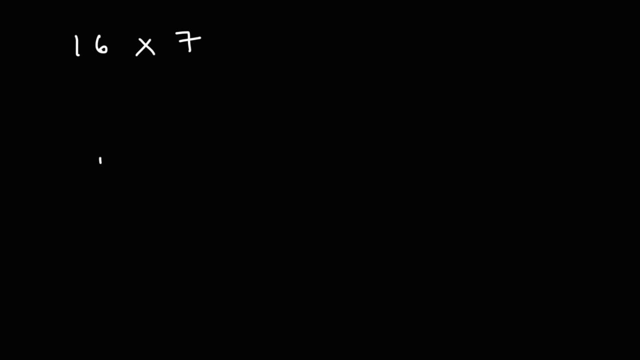 What is 16 times 7?? Well, one technique you can use is long multiplication. First, you can multiply 6 times 7. Which is 42. What you need to do is write the 2, carry over the 4.. 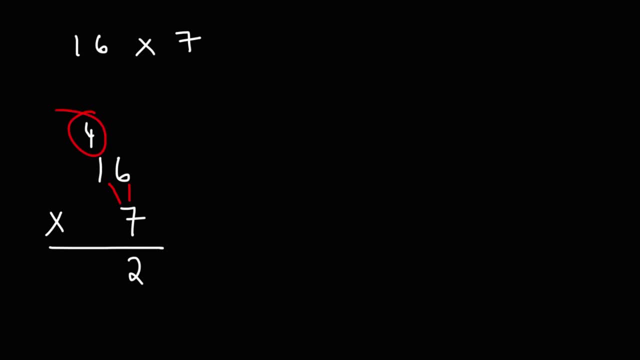 And then multiply 7 times 1,, which is 7., And then add the 4.. 7 plus 4 is 11.. Thus, 16 times 4 is 112.. Another way in which you could do this is you could break up 16 into two numbers. 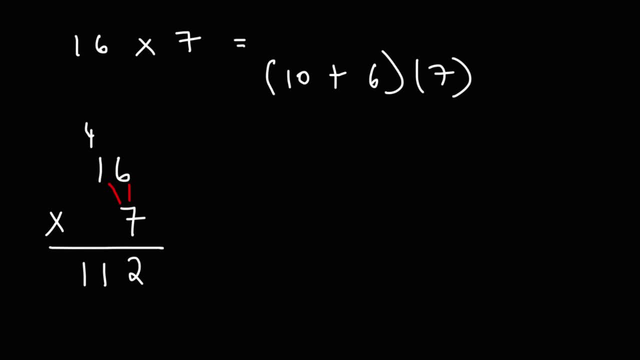 10 plus 6 is 16.. And then you could use the distributive property: 10 times 7. Is 70. And 7 times 6 is 42. And so you're adding 70 and 42 together. 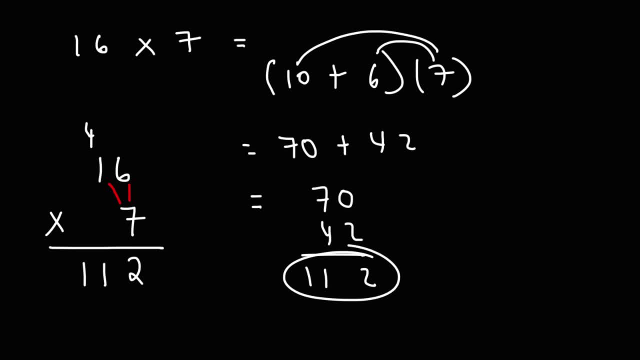 Which is 112.. So that's another way in which you can get the same answer. Now, what about 20 times 17?? What's the answer for that? Now, sometimes you could use money to represent math. If you had 17 $20 bills, how much money do you have? 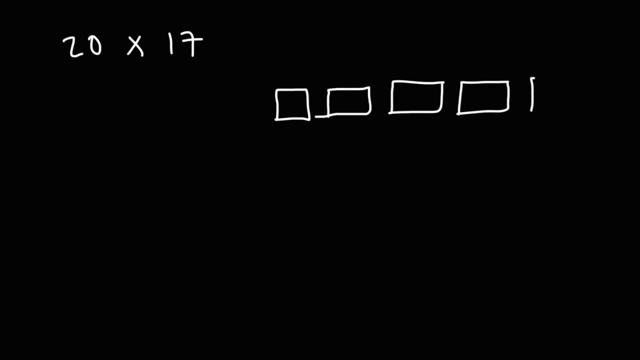 So imagine 5 $20 bills. 5 $20 bills corresponds to $100.. Now picture another 5 $20 bills, That's another $100.. And then picture another 5 $20 bills, That's 100 as well. 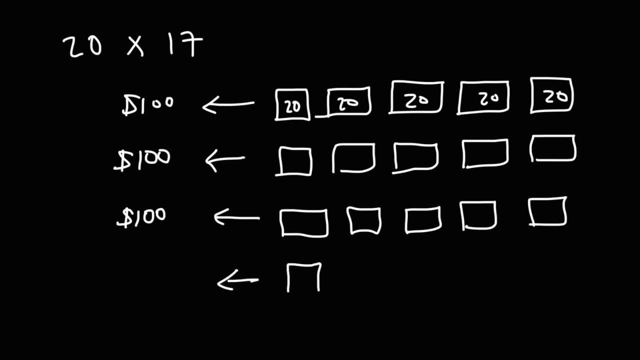 So right now we have 15 $20 bills. We need 17.. 2 $20 bills is 40.. So the total money you would have if you had 17 $20 bills is $340.. So 20 times 17 is 340.. 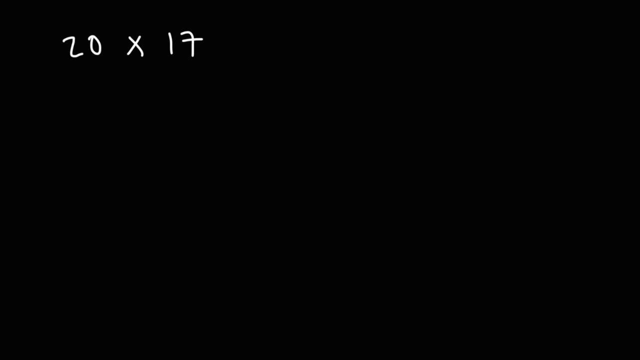 Now, sometimes you could use money to represent math If you had money. you could use money to represent math If you had 17 $20 bills. how much money do you have? So imagine five $20 bills. Five $20 bills corresponds to $100.. Now picture another five $20 bills. 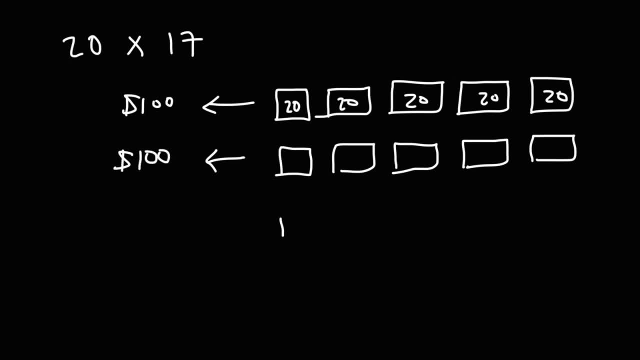 That's another $100.. And then picture another five $20 bills: That's another $100.. That's another $100 as well. So right now we have 15 $20 bills. We need 17.. Two $20 bills is 40.. 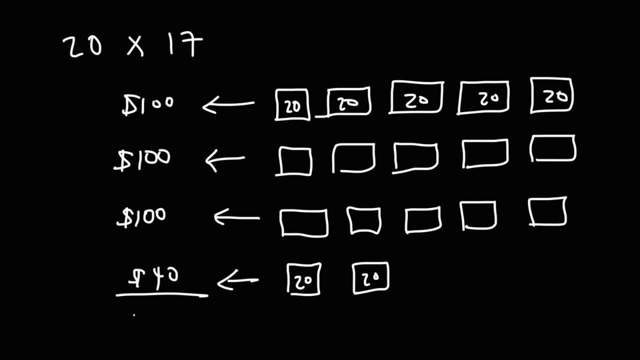 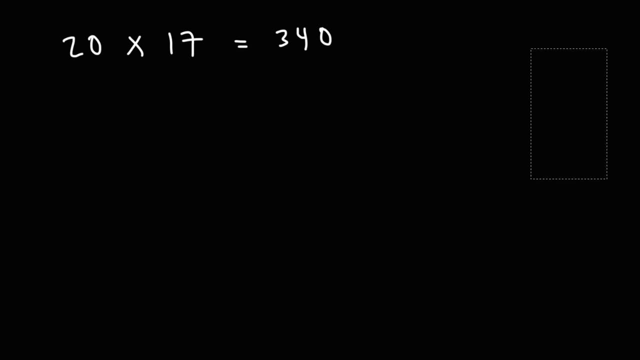 So the total money you would have if you had 17 $20 bills is $340.. So 20 times 17 is 340.. So you could use money to help you multiply. Let's add up two numbers. Now let's confirm our answer. 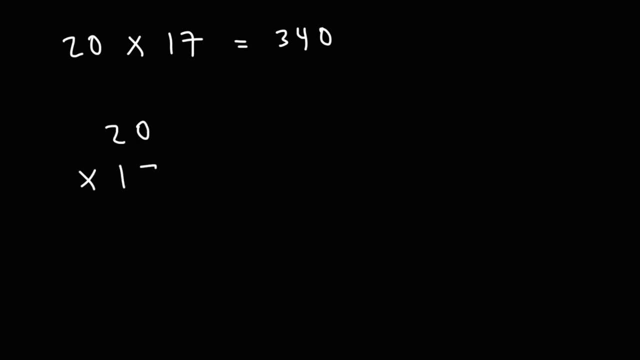 7 times 0 is 0. And then 7 times 2 is 14.. Now, before moving to the one, we need to add another zero. One times zero is zero, And then one times two is 340. And then one times two is 14.. 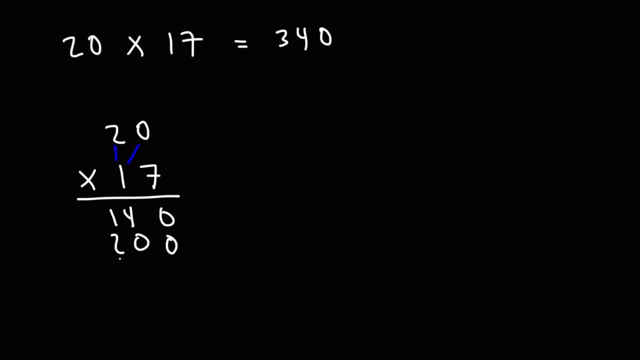 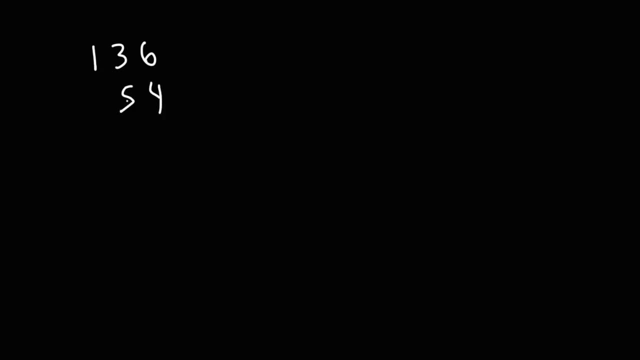 work on multiplying larger numbers. What's 136 times 54?? Feel free to pause the video if you want to work on this example. So first we're going to multiply 6 by 4.. 6 times 4 is 24.. We're. 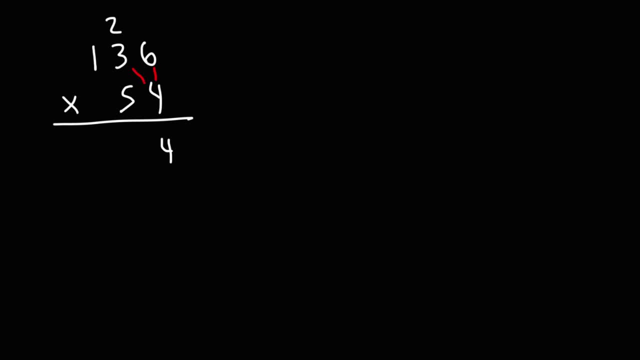 going to write the 4, carry over the 2.. And then 4 times 3 is 12, plus 2, that's 14.. So we'll write the 4, carry over the 1.. And then 4 times 1 is 4 plus 1, that's 5.. Next we're going to add a 0. 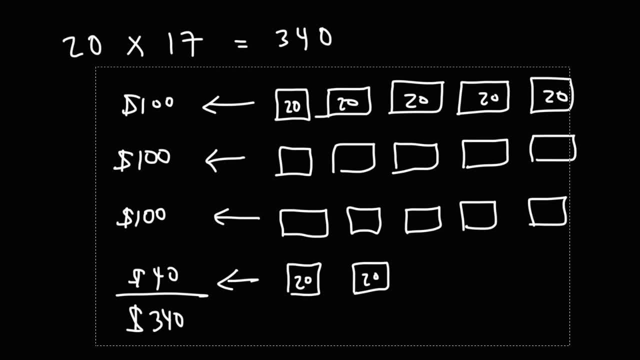 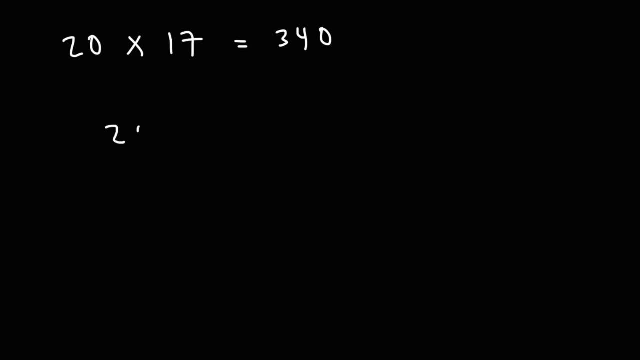 So you could use money to help you multiply two numbers. Now let's confirm our answer: 7 times 0 is 0. And then 7 times 2 is 14.. Now, before moving to the 1,, we need to add another 0.. 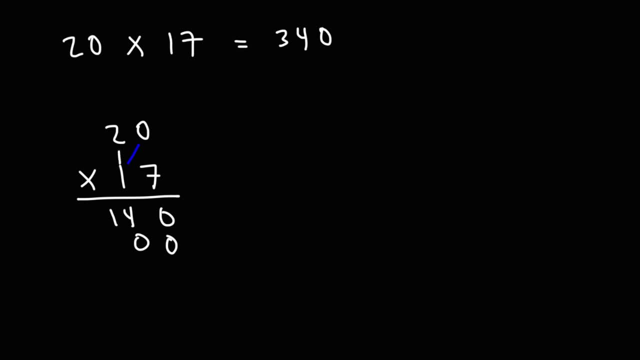 1 times 0 is 0.. And then 1 times 2,, that's 2.. And then we add 0 and 0 is 0.. 4 plus 0 is 4.. 2 plus 1 is 3.. 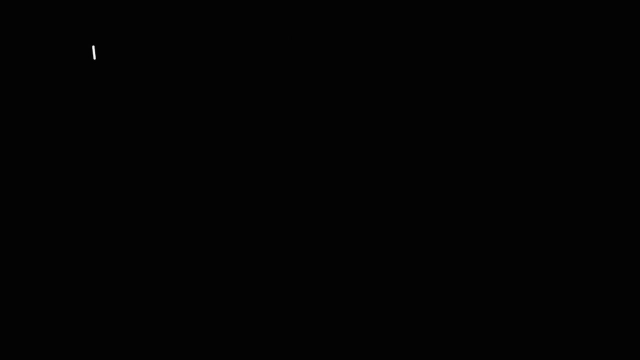 And so we get 340.. Now let's work on multiplying larger numbers. What's 136 times 54?? Feel free to pause the video if you want to work on this example. So first we're going to multiply 6 by 4.. 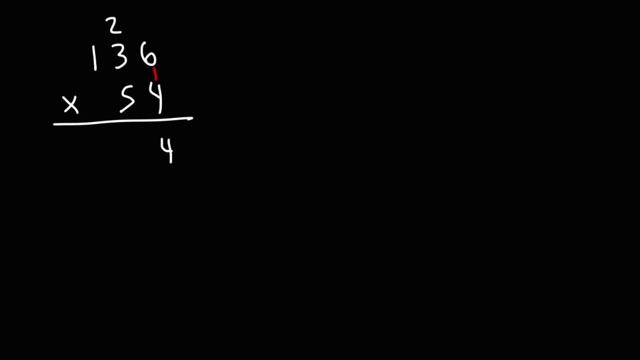 6 times 4 is 24.. We're going to write the 4, carry over the 2.. And then 4 times 3 is 12.. Plus 2, that's 14.. So we'll write the 4, carry over the 1.. 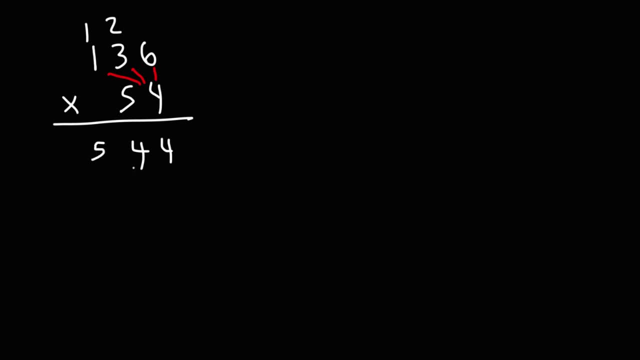 And then 4 times 1 is 4 plus 1, that's 5.. Next we're going to add a 0. And then we're going to multiply 5 and 6.. 5 times 6 is 30.. 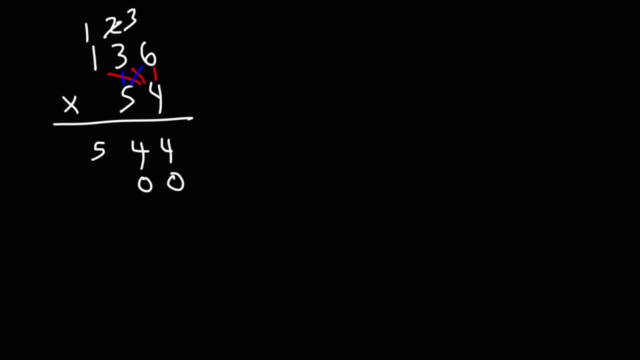 Carry over the 3.. And then 5 times 3 is 15, plus 3,, that's 18.. So we'll write the 8, carry over the 1. And then 5 times 1 is 5 plus 1, that's 6.. 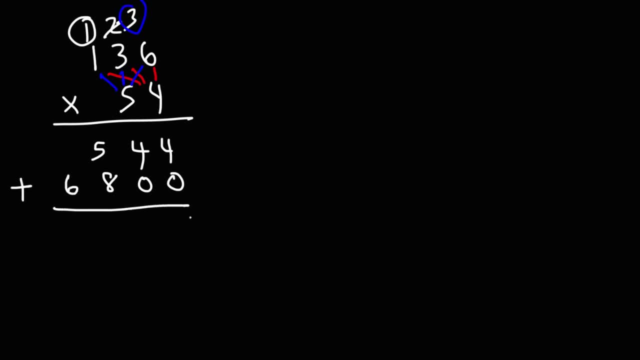 So this is what we get. Now we need to add 4 and 0 is 4.. 5 plus 8 is 13.. Carry over the 1. 6 plus 1 is 7.. So the answer is 7,344.. 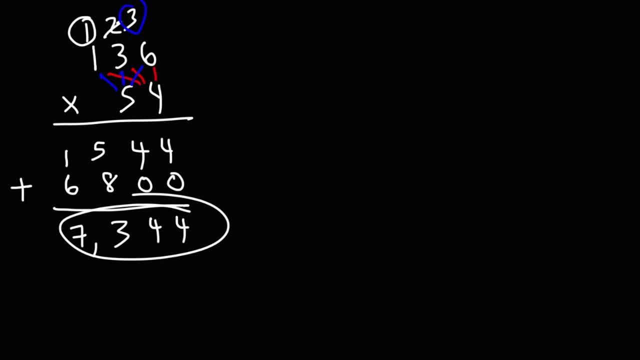 And of course, it's wise to confirm that with the calculator. So that answer is indeed correct. Now we're going to write the answer. Now, what about multiplying decimal numbers? What is 0.25 times 13?? Feel free to pause the video to work on that example. 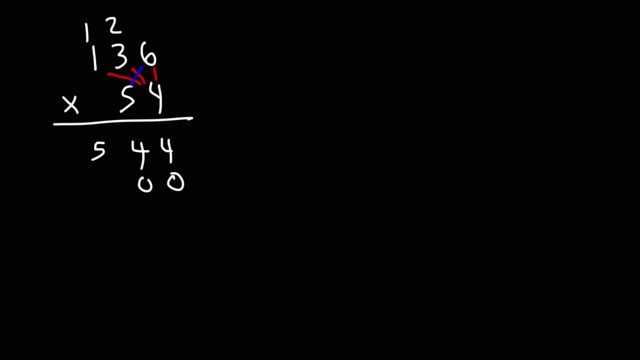 And then we're going to multiply 5 and 6.. 5 times 6 is 30,. carry over the 3.. And then 5 times 3 is 15, plus 3, that's 18.. So we'll write the 8,. 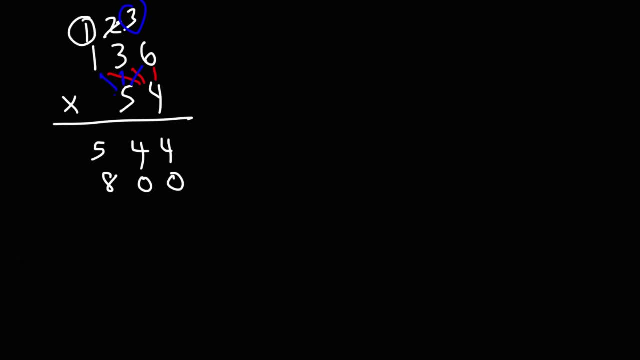 carry over the 1.. And then 5 times 1 is 5, plus 1,, that's 6.. So this is what we get Now. we need to add: 4 and 0 is 4.. 5 plus 8 is 13,. carry over the 1.. 6 plus 1 is 7.. So the answer is 7,344. 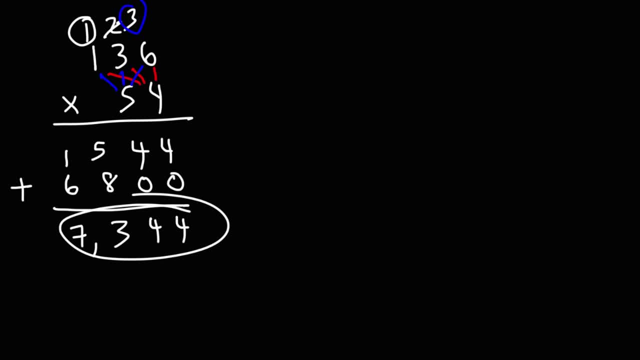 And of course it's wise to confirm that with the calculator. So that answer is indeed correct. Now what about multiplying decimal numbers? What is 0.25 times 13?? Feel free to pause the video to work on that example. Now for this one, we could use money to get the answer. Imagine having 13 quarters. 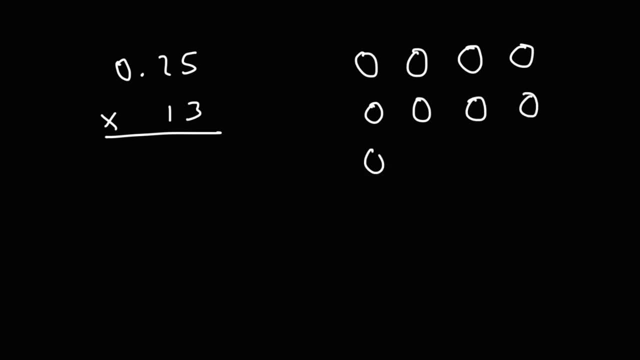 What is the value of money that you have Now? 4 quarters corresponds to a dollar, And right now we have a total of 12 quarters, So we need 1. one more. The last one is just worth $0.25.. So the total amount of money that we have is $3.25. 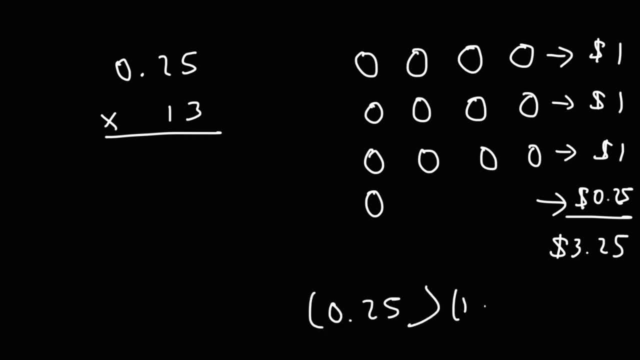 So we can say that 0.25 multiplied by 13 is 3.25.. Now let's confirm it. So we have 5 times 3, which is 15,, carry over the 1.. 2 times 3, which is 6, plus 1,, that's 7.. And 3 times 0 is 0,. 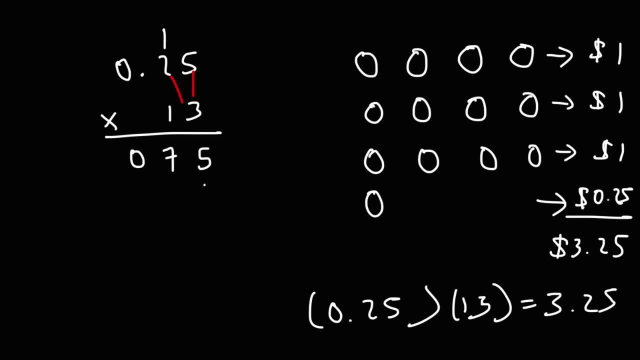 but you don't need to write that. You could, if you want to Now move it to the next row, add a 0.. Don't forget to do that. 1 times 5 is 5.. 1 times 2 is 2.. Don't worry about this one. 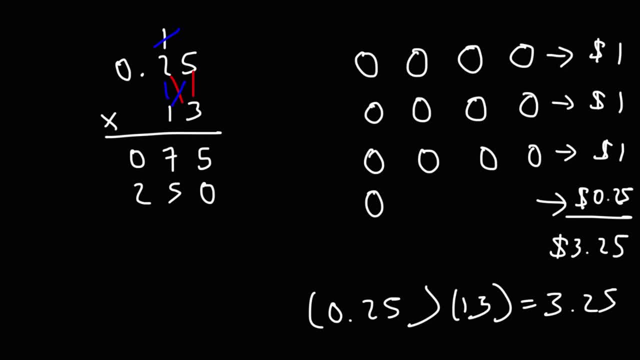 because we used that already And that's about it. So now we're going to add: 5 plus 0 is 5.. 5 plus 7 is 12, carry over the 1.. 1 plus 2 is 3.. 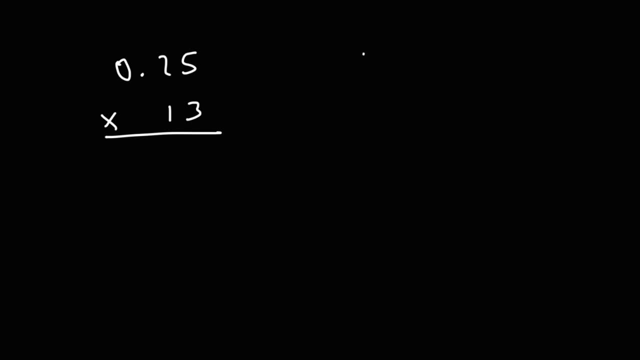 Now for this one. we could use money to get the answer. Imagine having 13 quarters. What is the value of money that you have Now? 4 quarters corresponds to a dollar, And right now we have a total of 12 quarters. 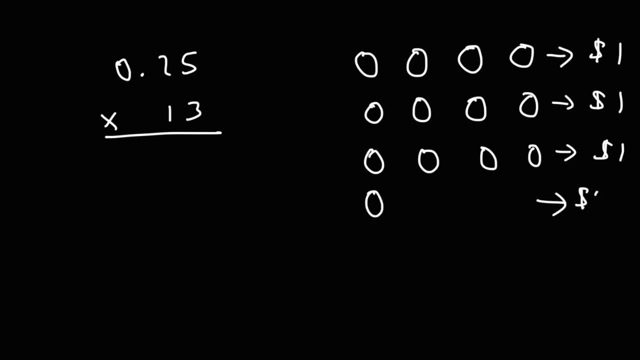 So we need one more. The last one is just worth 25 cents, So the total amount of money that we have is $3.25.. So we could say that 0.25 multiplied by 13 is 3.25.. 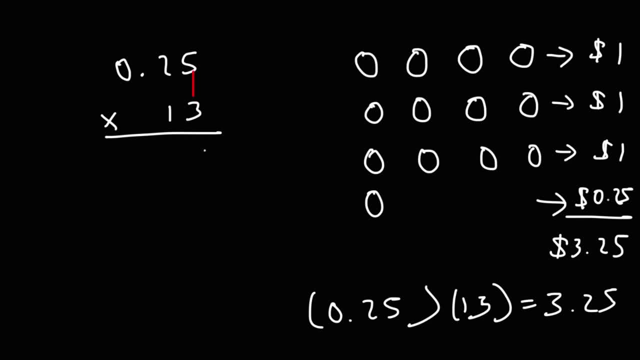 Now let's confirm it. So we have 5 times 3,, which is 15.. Carry over the 1.. 5 times 3,, which is 6,, plus 1,, that's 7.. And 3 times 0 is 0,. but you don't need to write that. 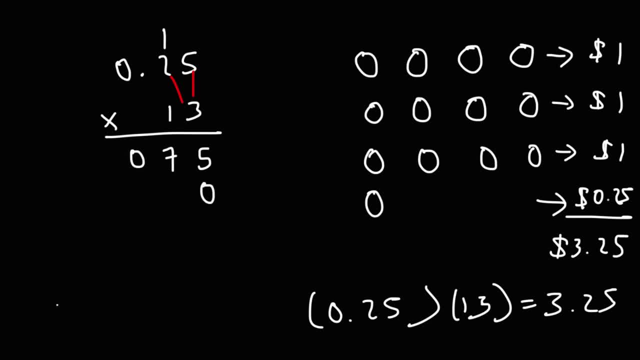 You could, if you want to Now, moving to the next row, add a 0.. Don't forget to do that. 1 times 5 is 5.. 1 times 2 is 2.. Don't worry about this one, because we used that already. 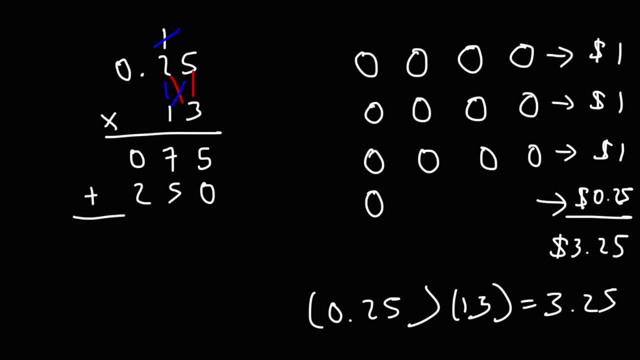 And that's about it. So now we're going to add: 5 plus 0 is 5.. 5 plus 7 is 12.. Carry over the 1.. 1 plus 2 is 3.. Now notice that we have two numbers to the right of this decimal. 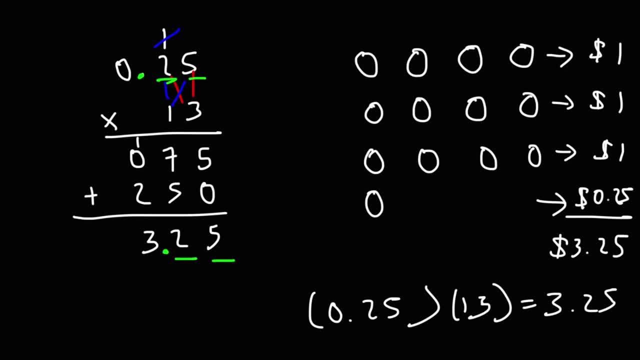 So in our answer we're going to have two numbers to the right of the decimal. Therefore the answer is 3.25.. So that's how you can multiply decimal numbers And that's how you can use money to illustrate the math problem and even get the answer. 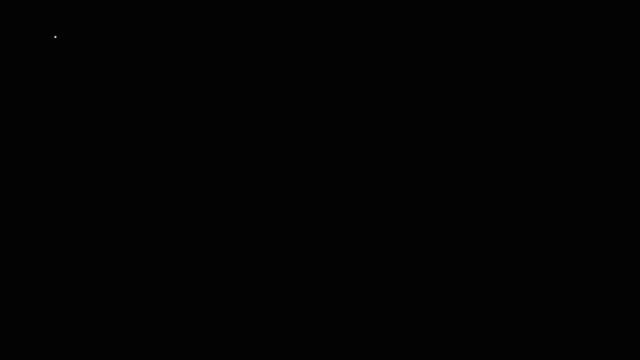 Now let's take a look at the next row. Now let's move on to multiplying certain types of large numbers. 10 times 10 is 100.. 10 times 100 is 1000.. And here's a simple way to get the answer. 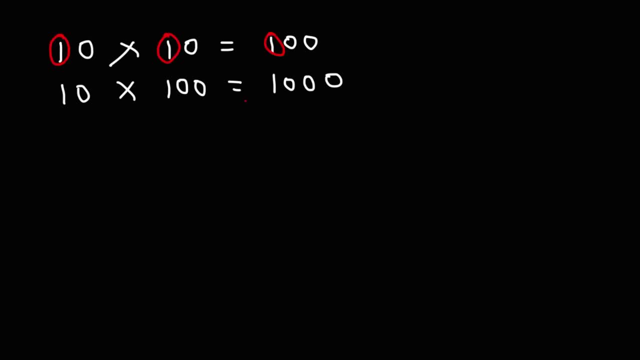 If you multiply 1 by 1,, you get 1.. And then you need to add the zeros. Here we have two zeros on the left. The final answer will contain two zeros. For 10 times 100,, we have a total of three zeros. 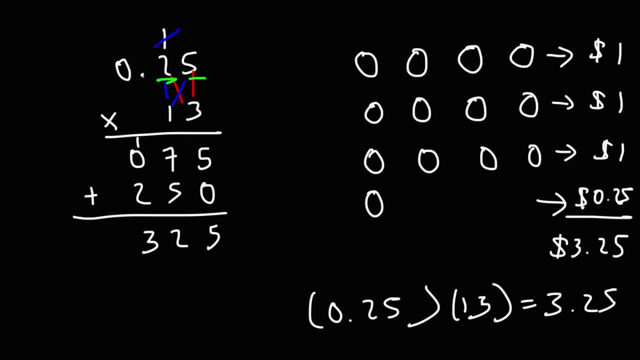 Now notice that we have two numbers to the right of this decimal. So in our answer we're going to have two numbers to the right of the decimal. Therefore the answer is 3.25.. So that's how you can multiply decimal numbers And that's how you can use money to illustrate the math problem and 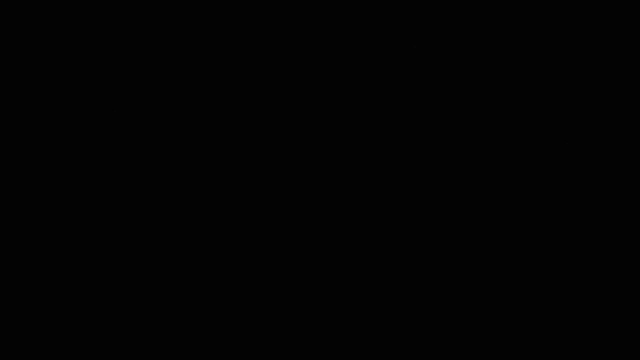 even get the answer. Now let's move on to multiplying certain types of large numbers. 10 times 10, is 100.. 10 times 100, is 1000.. And here's a simple way to get the answer: If you multiply 1 by 1,, 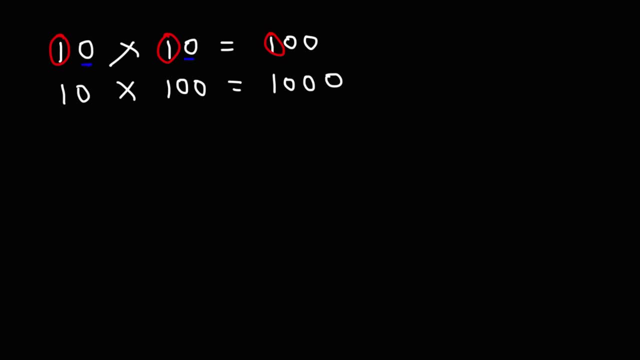 you get 1.. And then you need to add the zeros. Here we have two zeros on the left. The final answer will contain two zeros. For 10 times 100, we have a total of three zeros. So the final answer has three zeros as well. 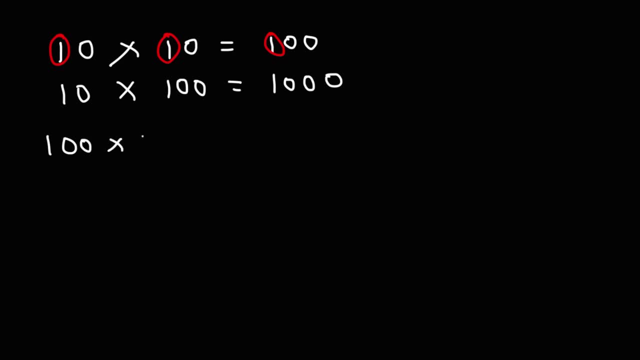 So let's say, if we want to multiply 100 by 100.. What I would do is multiply 1 by 1, which is 1, and then add the number of zeros that we have. We have a total of four zeros. 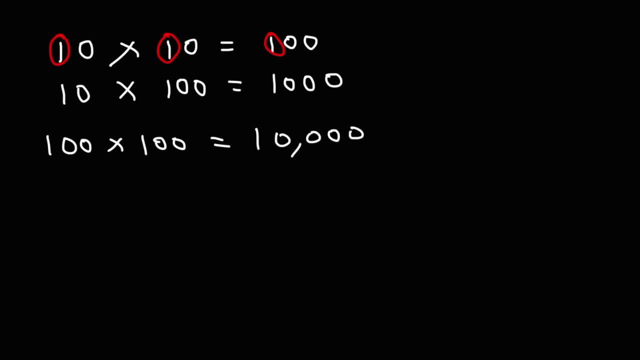 So then I would just write the four zeros, So the answer is 10,000.. Based on that, what is 50 times 100?? Well, 5 times 1 is 5.. And then we have a total of three zeros, So the answer is 10,000. 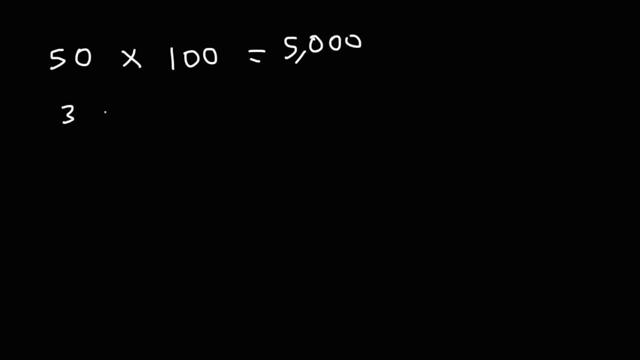 the answer is 5,000.. If we want to multiply 30 by 200,, I would multiply 3 by 2, that's 6, and then write the three zeros. So the answer is 6,000.. Now, if I want to multiply, 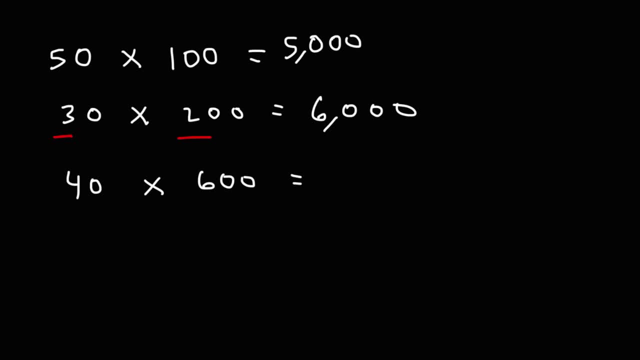 40 by 600,, this will be 4 times 6,, which is 24, and then add the three zeros, So the answer is 24,000.. What about these two? 700 times 800, and also 3,000 times 5,000.. 7 times 8. 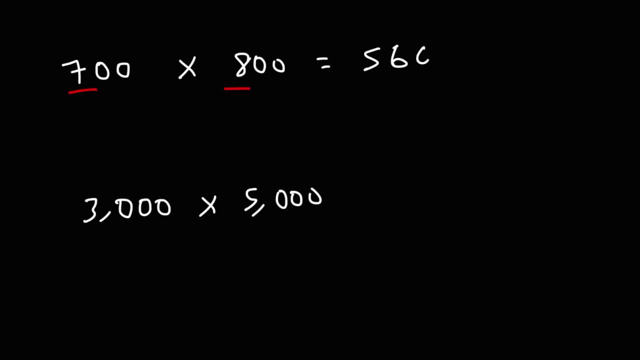 is 56, and we have a total of four zeros. So this is going to be 560,000.. 3,000 times 5,000, we can multiply 3 and 5 to get 15, and then we can multiply 3 and 5 to get 15,. 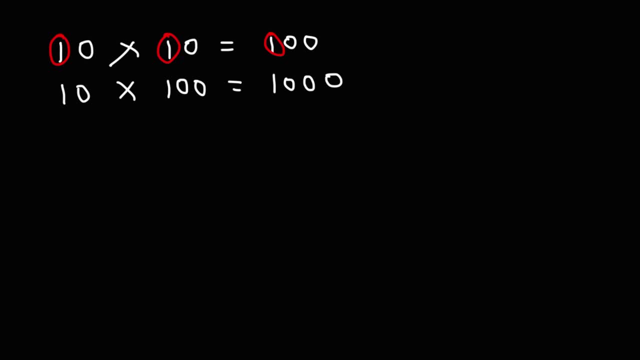 So the final answer has three zeros as well. So let's say, if we want to multiply 100 by 100.. What I would do is multiply 1 by 1, which is 1.. And then add the number of zeros that we have. 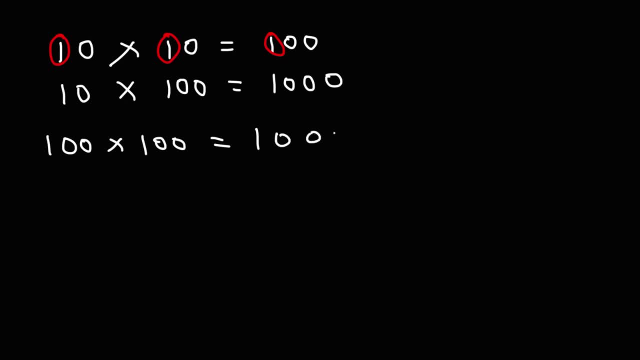 We have a total of four zeros. So then I would just write the four zeros. So the answer is 10,000.. Based on that, what is 50 times 100?? Well, 5 times 1 is 5.. 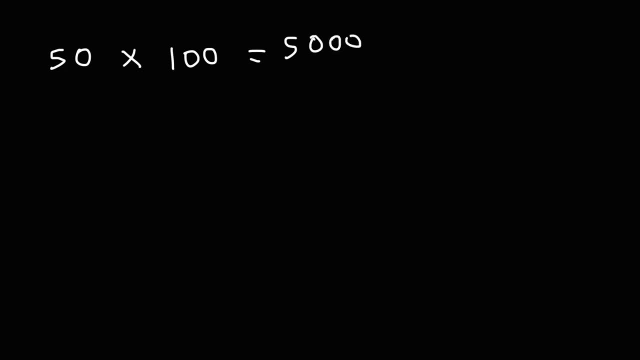 And then we have a total of three zeros. So the answer is 5,000.. If we want to multiply 30 by 200, I would multiply 3 by 2.. That's 6.. And then write the three zeros. 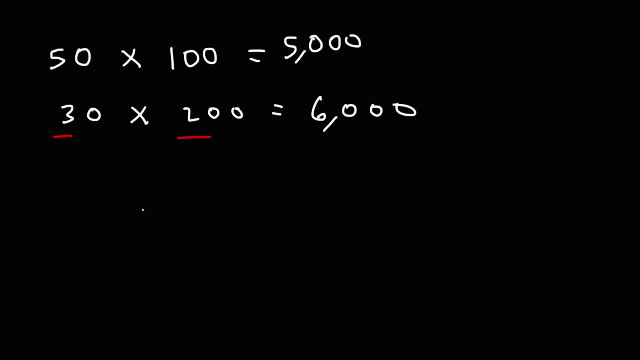 So the answer is 6,000.. Now, if I want to multiply 40 by 600, this will be 4 times 6,, which is 24.. And then add the three zeros, So the answer is 24,000.. 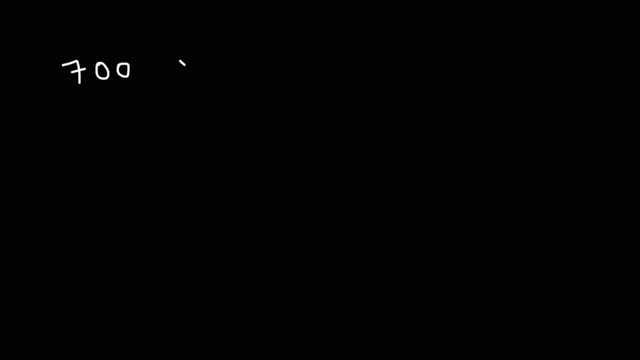 What about these two? 700 times 800.. And also 3,000 times 5,000.. 7 times 8 is 56. And we have a total of four zeros. So this is going to be 506.. 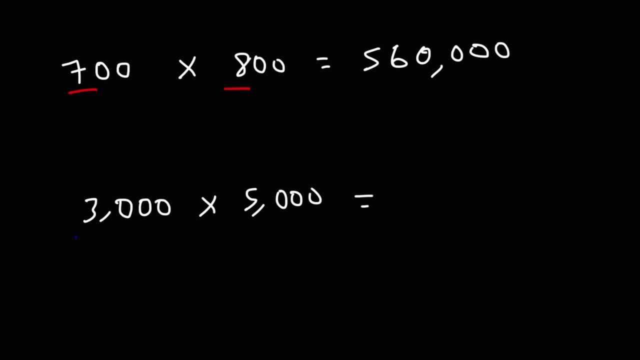 3,000 times 5,000.. We can multiply 3 and 5 to get 15.. And then we have a total of six zeros. So the answer is going to be 15,000,000.. So that's how you can multiply large numbers. 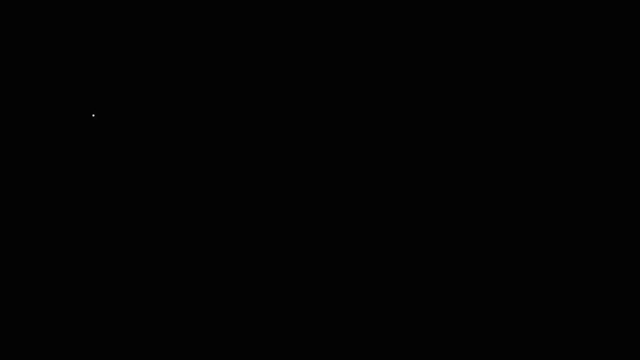 Now let's say, for instance, you want to multiply 598 by, let's say, 802.. So for something like this, if you want to get a quick estimate of what the answer is, you can round 598 to 600.. 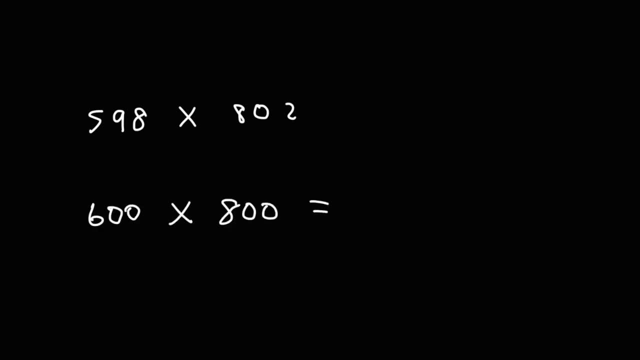 And you can round 802 to 800. And so 6 times 8 is 48. And then you can carry the four zeros. So the answer is going to be close to 480,000.. Now let's get the exact answer. 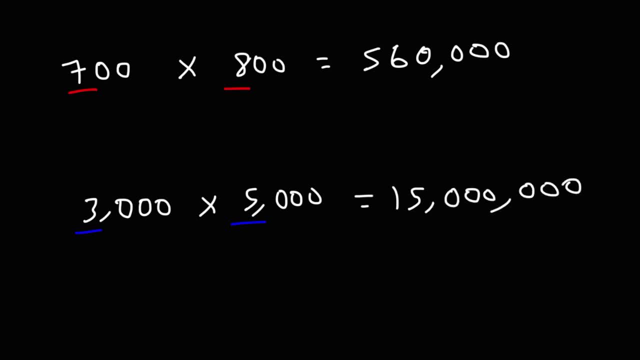 and then we can multiply 3 and 5 to get 15,, and then we can multiply 3 and 5 to get 15,, and then we have a total of six zeros. So the answer is going to be 15,000,000.. So that's. 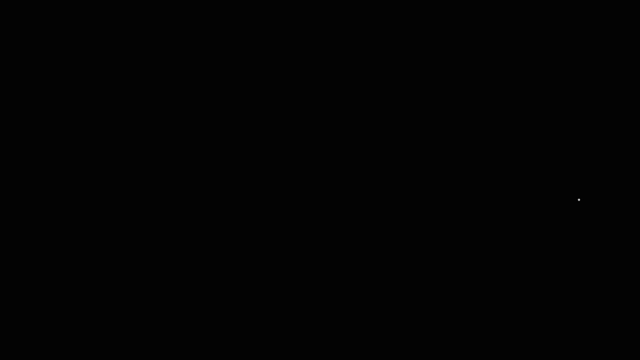 how you can multiply large numbers. Now let's say, for instance, you want to multiply 598 by, let's say, 802.. So for something like this, if you want to get a quick estimate of what the answer is, you can round 598 to 600, and you can round 802 to 600, and you 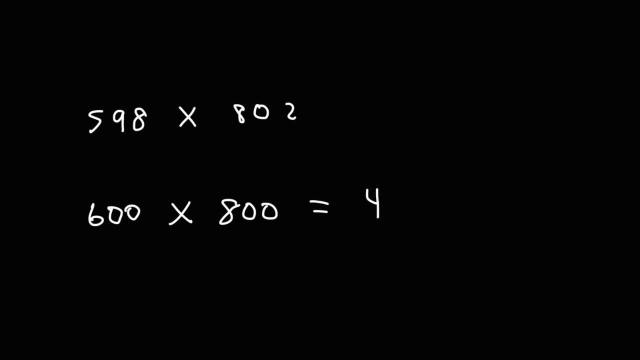 can round 802 to 800.. And so 6 times 8 is 48, and then you can carry the four zeros. So the answer is going to be close to 480,000.. Now let's get the exact answer: 598 times. 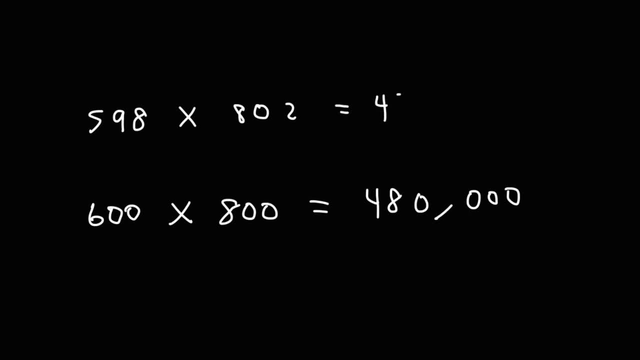 802.. The exact answer is 479,596.. So when dealing with large numbers, if you need to estimate the answer, this technique is very useful. Now let's talk about division. Let's say, if we want to divide 63 by 9.. How can we find the answer? Now, what you need to know. 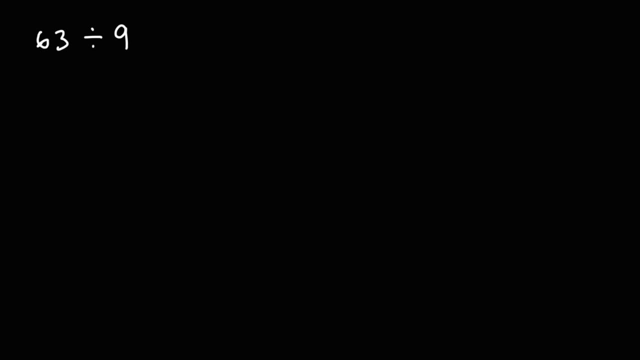 is that division is the opposite of multiplication. By the way, you can also rewrite this problem like this: as a fraction. So 63 over 9 is the same as 63 divided by 9.. Now to find the answer, ask yourself 9 times what number. 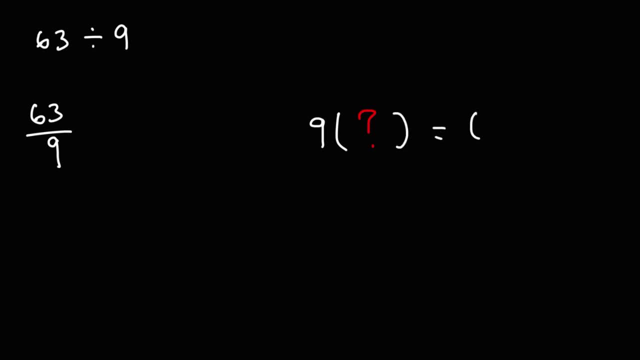 is equal to 63. And this is one of those situations where it would help you if you know the multiplication table. So, 9 times what number is 63?? So, using the multiplication table, 9 times 7 is 63. Therefore, 63 divided by 9 is 7.. And so that's how you could divide numbers. 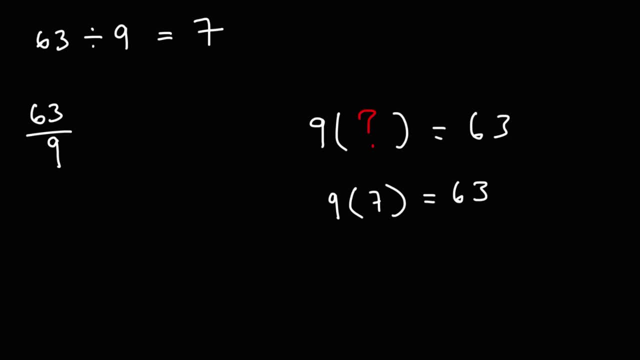 If you know your multiplication table, you can use that to find the answer to division problems like these. So here's another example. Let's say we want to find 36 divided by 4, which is the same as 36 over 4.. What is the answer? So, 4 times what number? 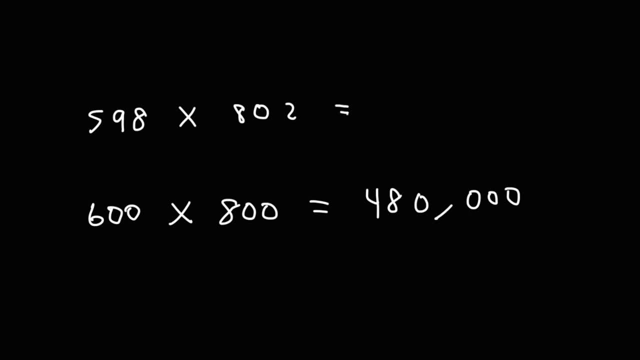 598 times 802.. The exact answer is 479,596.. So when dealing with large numbers, if you need to estimate the answer, this technique is very useful. Now let's talk about division. Let's say, if we want to divide 63 by 9.. 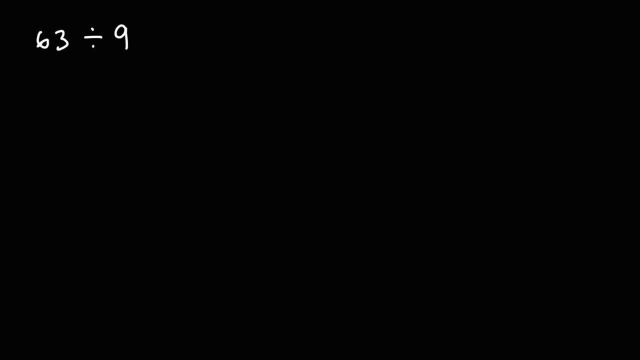 How can we find the answer Now? what you need to know is that division is the opposite of multiplication. By the way, you can also rewrite this problem like this as a fraction. So 63 over 9 is the same as 63 divided by 9.. 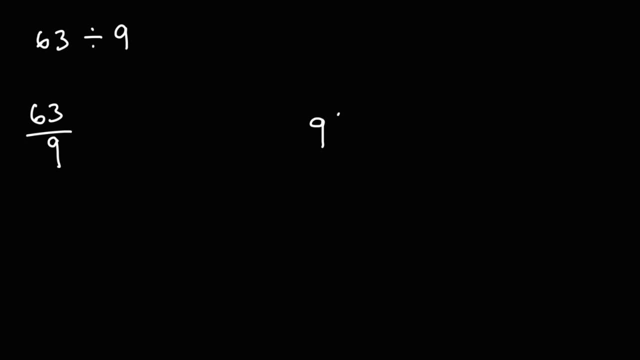 Now to find the answer. ask yourself: 9 times, what number is equal to 63?? And this is one of those situations where it would help you if you know the multiplication table. So, 9 times what number is 63?? 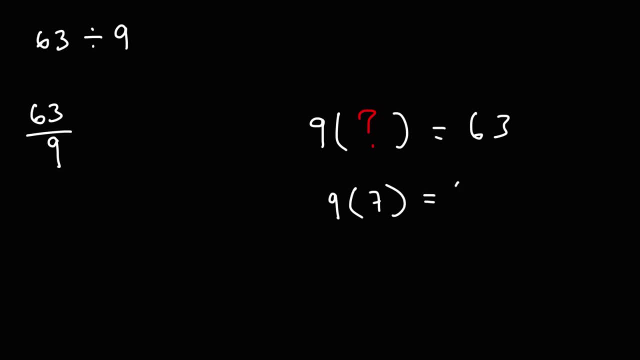 So, using the multiplication table, 9 times 7 is 63. Therefore, 63 divided by 9 is 7.. And so that's how you could divide numbers. If you know your multiplication table, you can use that to find the answer. 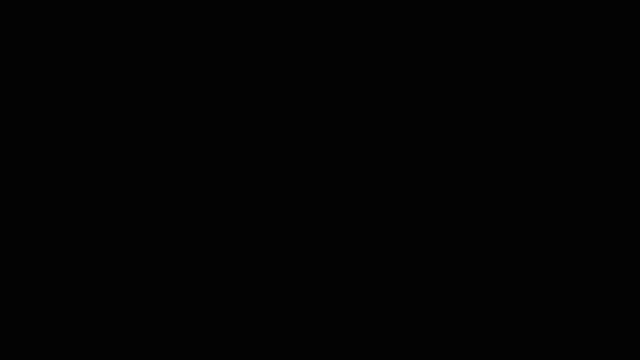 to division problems like these. So here's another example. Let's say we want to find 36 divided by 4, which is the same as 36 over 4.. What is the answer? So 4 times what number is 36?? 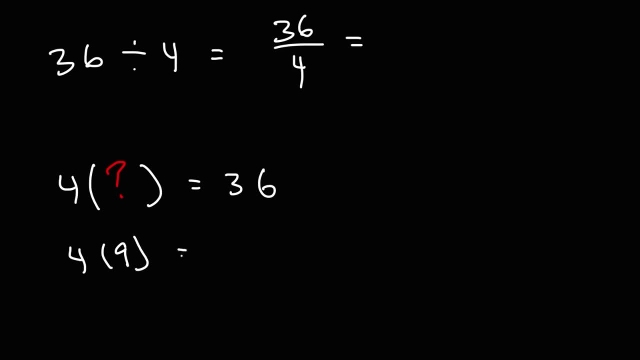 That's the question. Well, we know that 4 times 9 is 36.. So 36 divided by 4 is 9.. Now what about 28 divided by 4? What's the answer? 4 times what number is 28?? 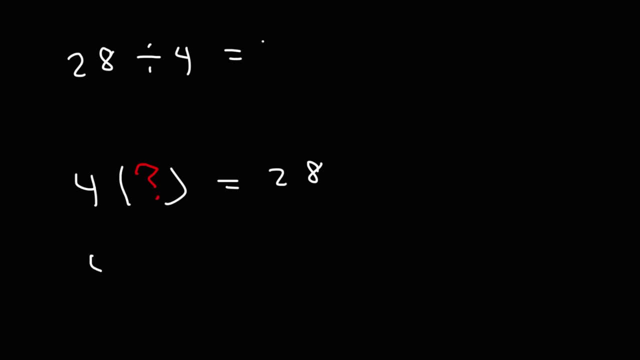 The answer is 7.. 4 times 7 is 28.. So 28 divided by 4 is 7. And that's how you could perform basic division. Now let's work on some examples where we're using larger numbers. 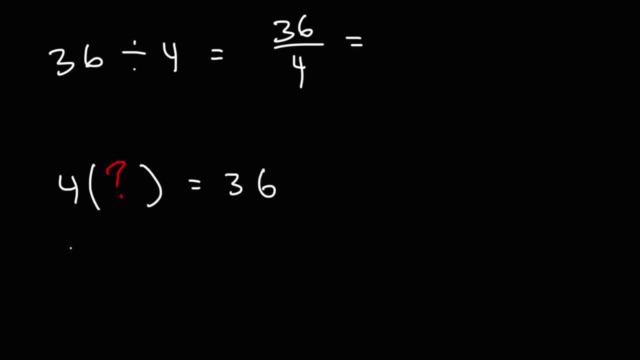 is 36?? That's the question. Well, we know that 4 times 9 is 36.. So 36 divided by 4 is 9.. Now, what about 28 divided by 4? What's the answer? 4 times what number is 28? The answer is 7.. 4 times 7 is 28.. So 28 divided by 4 is 7.. 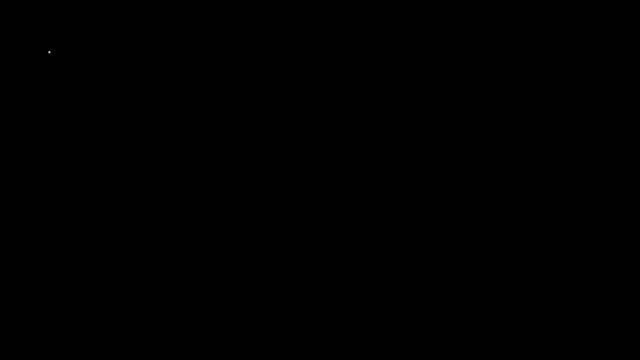 And that's how you could perform basic division. Now let's work on some examples where we're using larger numbers. Let's say, if we wanted to divide 200 by 5. What is the answer? Well, it helps to think of 200 as 20 times 10.. 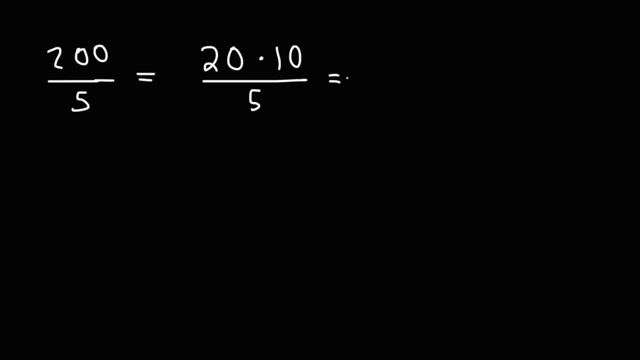 10 divided by 5 is 2.. So what we have left over is 20 times 2.. And then 20 times 2 is 40. So 200 divided by 5 is 40. That's one way you could do it. 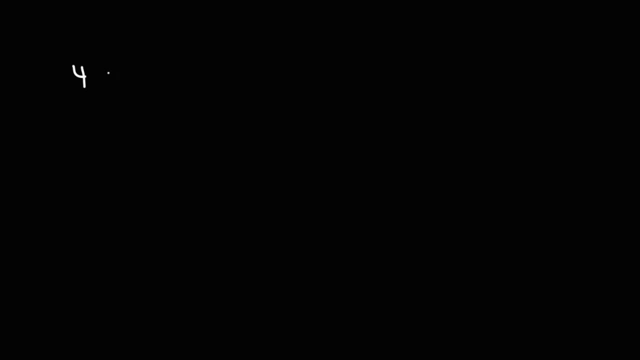 Let's work on another example: 4200 divided by 7.. What's the answer? Well, 4200,. you could write that as 42 times 100.. And then 42 divided by 7 is 6.. So you have 6 times 100, which. 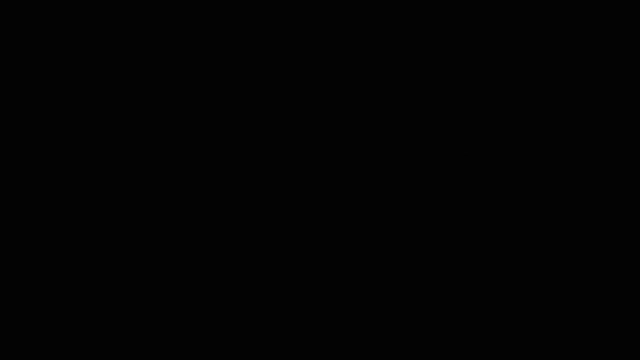 is 600.. So that's the answer for that one. Now, what about 24,000 divided by 40?? If you see this, the first thing I would recommend doing is canceling a zero. So this becomes 2400 divided by 4.. 2400 is 24 times 100. And 24 divided by 4 is 6.. So you have 6 times 100,. 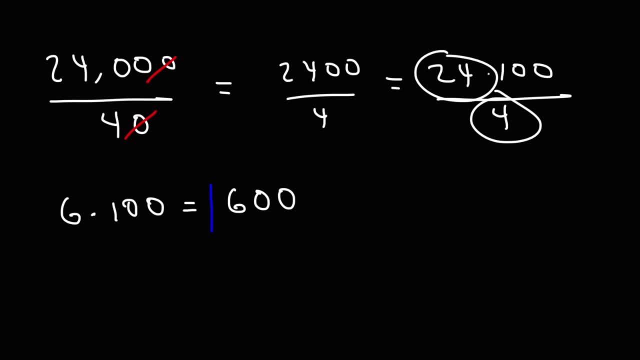 giving us the final answer of 600.. Let's work on one more example. Let's divide 3500 by 500.. So, like before, we could cancel zeros, So we can cancel two zeros, on the top and on the bottom. So this is 35 divided by 5, which is simply 7.. Actually, let's work on one more. 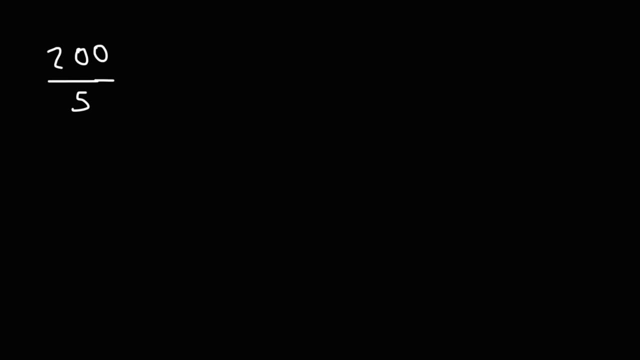 Let's say if we wanted to divide 200 by 5.. What is the answer? Well, it helps to think of 200 as 20 times 10.. 10 divided by 5 is 2.. So what we have left over is 20 times 2.. 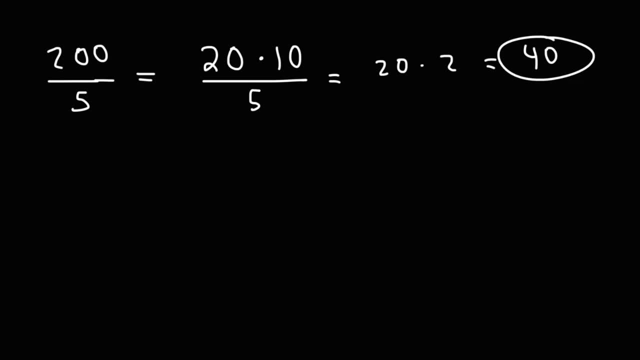 And then 20 times 2 is 40. So 200 divided by 5 is 40. That's one way you could do it. Let's work on another example: 4200 divided by 7.. What's the answer? 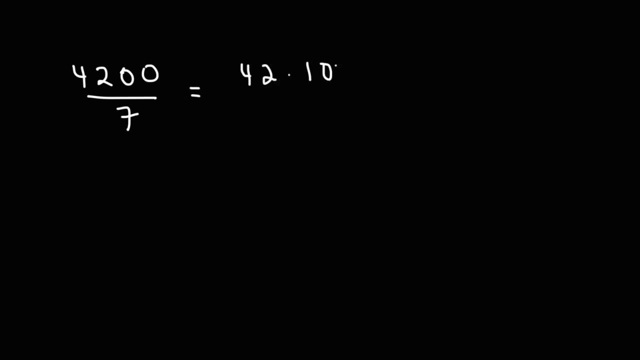 Well, 4200,. you could write that as 42 times 100. And then 42 divided by 7 is 6.. So you have 6 times 100, which is 600.. So that's the answer for that one. 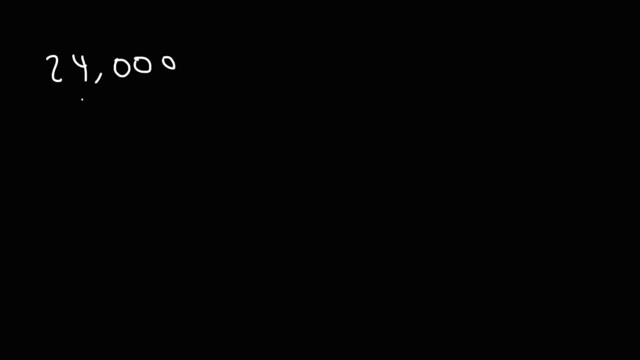 Now, what about 24000 divided by 40?? If you see this, the first thing I would recommend doing is cancelling a 0.. So this becomes 2400 divided by 4.. 2400 is 24 times 100.. 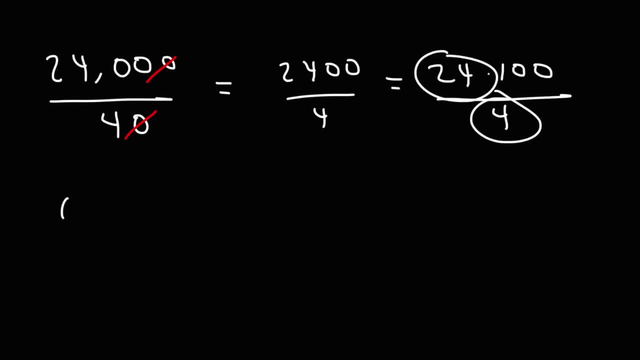 And 24 divided by 4 is 6.. So you have 6 times 100, giving us the final answer of 600.. Let's work on one more example. Let's divide 3500 by 500.. So, like before, we could cancel 0s. 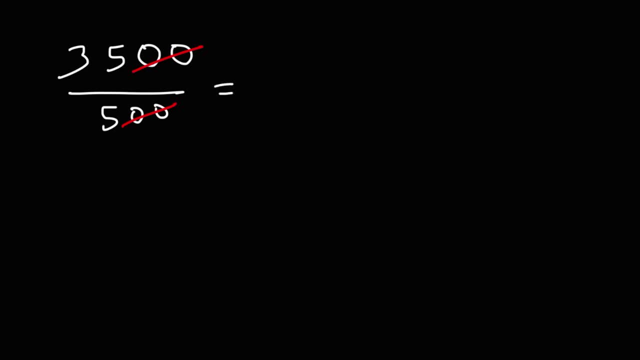 So we can cancel two 0s, on the top and on the bottom. So this is 35 divided by 5, which is simply 7.. Actually, let's work on one more example, but this time with a much larger number. 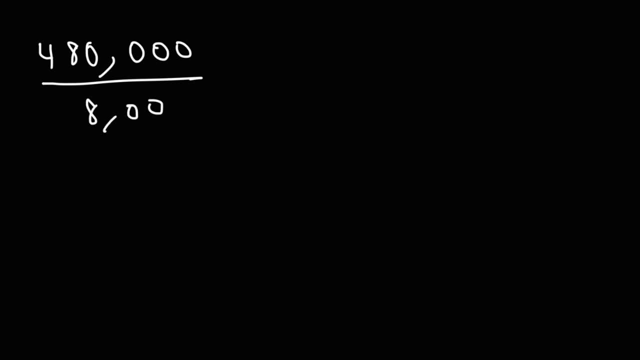 Let's divide 480000 by 8000.. In this example we can cancel three 0s, So this becomes 480 divided by 8.. 480, we can break that down into 48 times 10. And 48 divided by 8 is 6.. 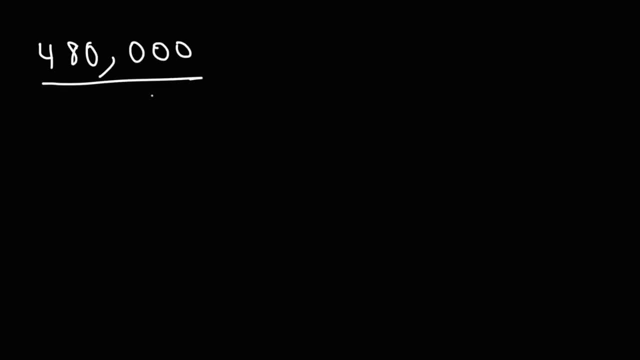 example, but this time with a much larger number. Let's divide 480,000 by 8,000.. In this example we can cancel three zeros. So this is 480,000 divided by 8,000.. And this becomes 480 divided by 8.. 480, we can break that down into 48 times 10.. And 48 divided 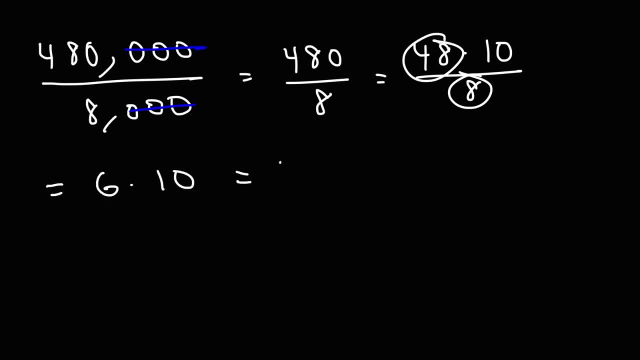 by 8 is 6.. And 6 times 10 is 60.. So that's how you could divide large numbers. Now, what about this example? Let's say, if we want to divide 38 by 5.. 5 doesn't go evenly into 38.. 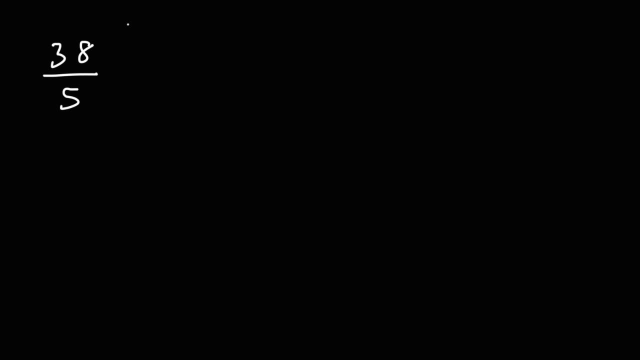 In this case we're going to get a decimal. It's known as an improper fraction. To convert the improper fraction into a decimal you could use long division. So 5 go into 38. seven times 5 times 7 is 35.. 38 minus 35 is 3.. 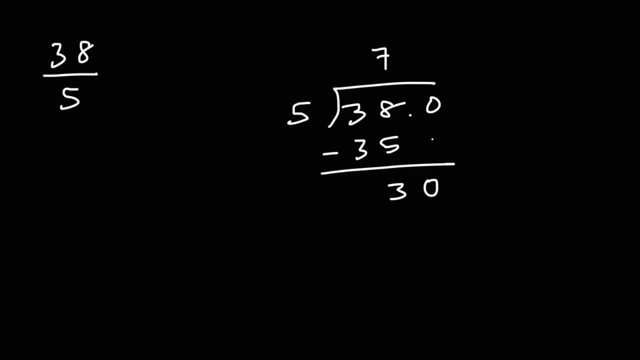 Now what's going to add is 0.. 5,. since we added a decimal point, we need to add it here as well. 5 goes into 30.. 6 times 5 times 6 is 30.. So 5 times 0.6 is 3.0.. And so the remainder is 0.. Thus 38 divided by: 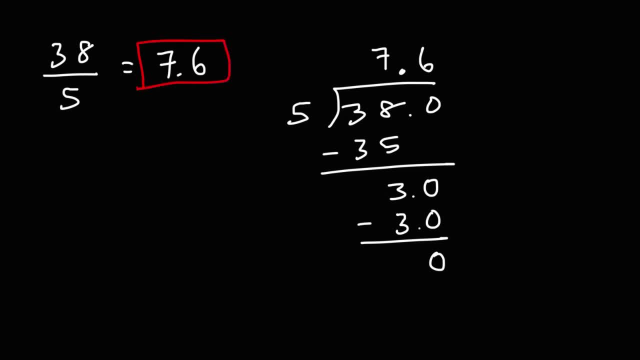 5 is 7.6.. Let's consider some more examples. Let's say, if we want to divide 43 by 8.. Go ahead and work on that example. So first we need to determine how many times does 8 go into 43.? 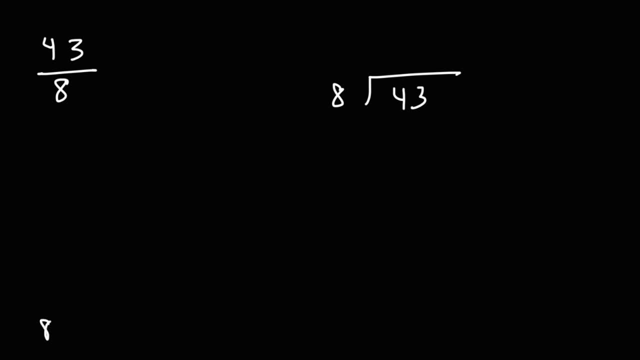 It helps to write down the multiples of 8, which I'll do over here. So we have 8,, 16,, 24,, 32,, 40,, 48,, 56,, 64.. And I'll stop it there. 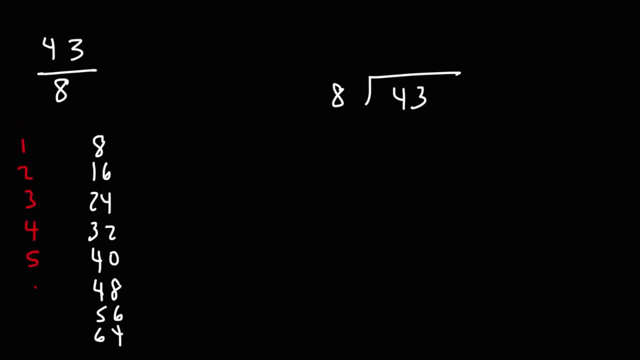 8 times 2 is 16.. 8 times 3 is 24. And so forth. So what you want to do is choose the highest multiple of 8 just under 43. And that is going to be 40. So 8 goes into 43 five times. 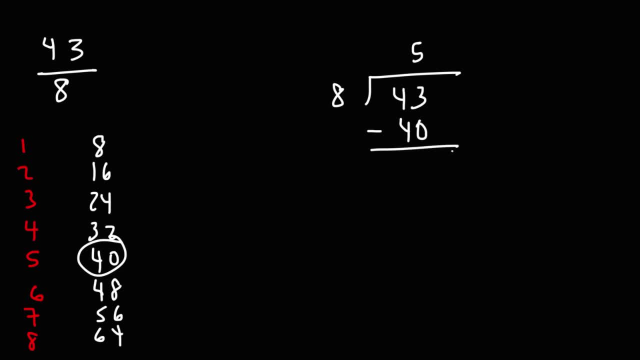 8 times 5 is 40. Subtract the two numbers, you get 3.. Now 8 doesn't go into 3, so we need to add a decimal point And add a 0. So how many times does 8 go into 30?? 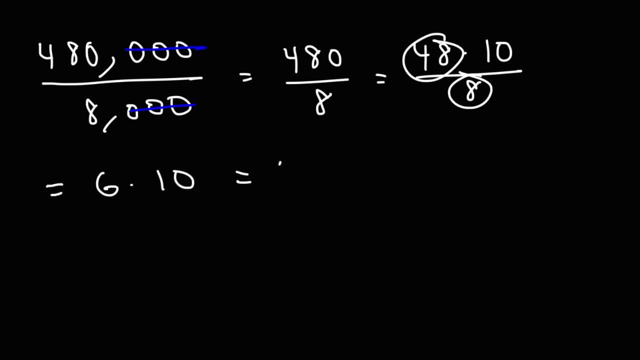 And 6 times 10 is 60.. So that's how you can divide large numbers. Now, what about this example? Let's say, if we want to divide 38 by 5.. 5 doesn't go evenly into 38.. 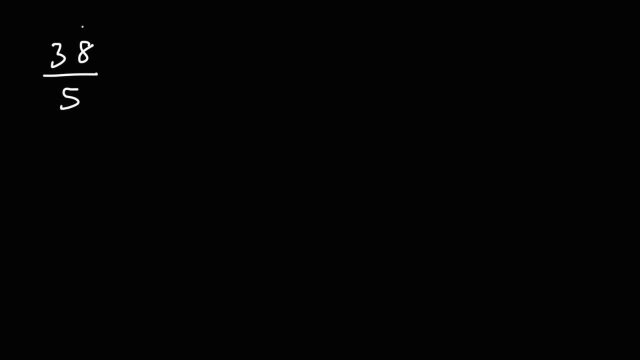 In this case we're going to get a decimal. This is also known as an improper fraction. To convert the improper fraction into a decimal you could use long division. So 5 goes into 38. seven times 5 times 7 is 35.. 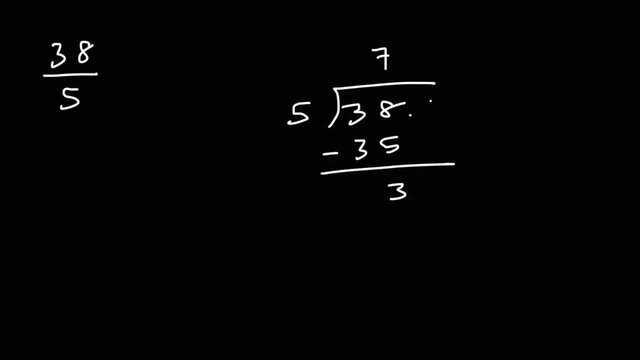 38 minus 35 is 3.. Now what's good to add is 0.. 5,. since we added a decimal point, we need to add it here as well. 5 goes into 30. six times 5 times 6 is 30, so 5 times 0.6 is 3.0.. 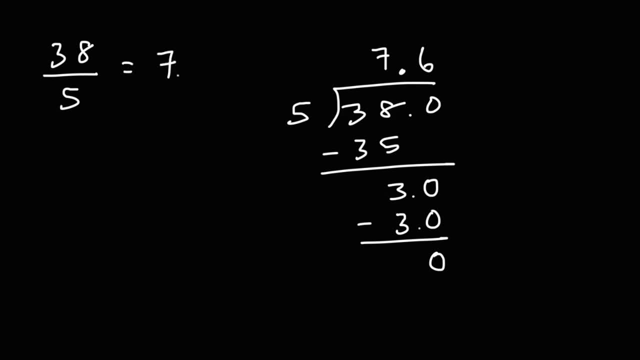 And so the remainder is 0. Thus, 38 divided by 5 is 7.6.. Let's consider some more examples. Let's say, if we want to divide 43 by 8. Go ahead and work on that example. 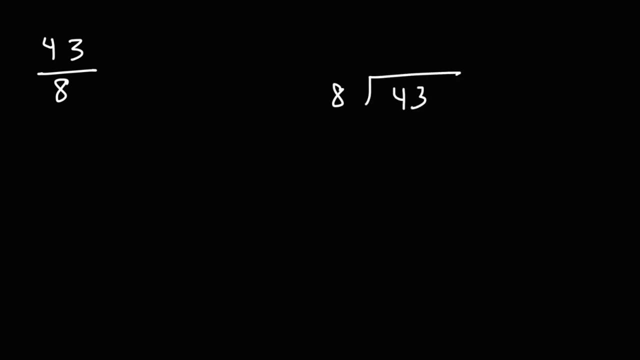 So first we need to determine how many times does 8 go into 43. It helps to write down the multiples of 8, which I'll do over here. So we have 8,, 16,, 24,, 32,, 40,. 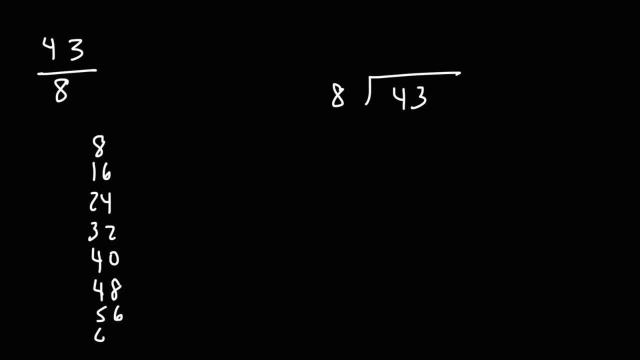 48,, 56,, 64.. And I'll stop it there: 8 times 2 is 16,, 8 times 3 is 24, and so forth. So what you want to do is choose the highest multiple of 8, just under 43.. 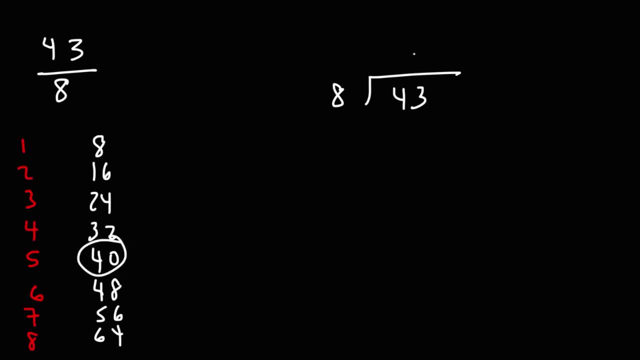 And that is going to be 40.. So 8 goes into 43. five times 8 times 5 is 40.. Subtract the two numbers, you get 3.. Now 8 doesn't go into 3.. So we need to add a decimal point and add a 0. 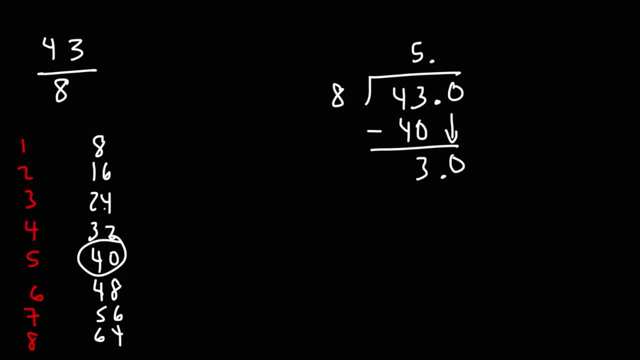 So how many times does 8 go into 30? 8 goes into 30 three times. If 8 times 3 is 24,, 8 times 0.3 is 2.4.. Subtracting these two numbers, we get 0.6.. 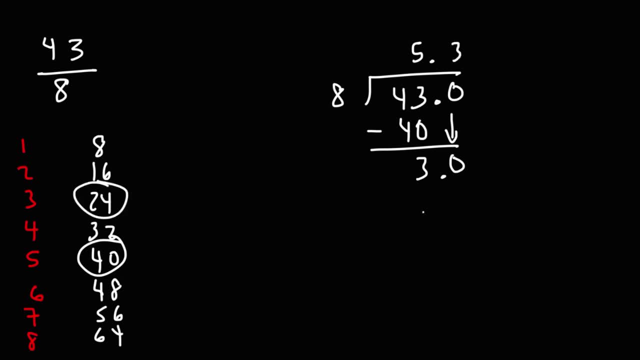 8 goes into 30 three times. If 8 times 3 is 24, 8 times 0.3 is 2.4.. Subtracting these two numbers, we get 0.6.. Next we need to add another 0.. 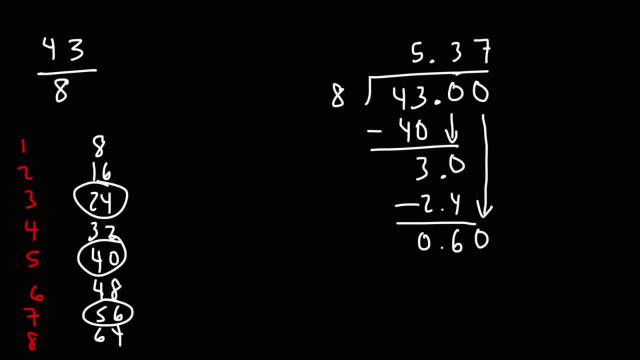 8 goes into 60 seven times 8 goes into 60. seven times 8 times 7 is 56. So the difference between 60 and 56 is 4.. Add another 0.. 8 goes into 40 five times. 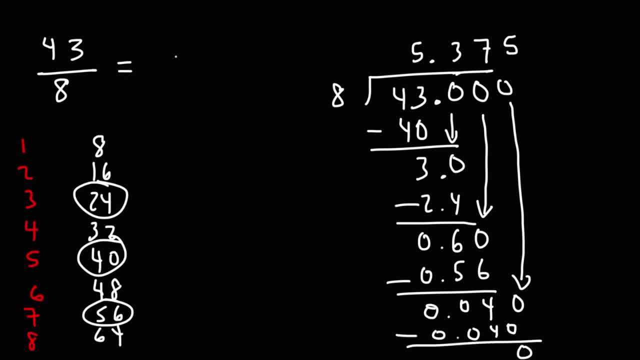 And this gives us a remainder of 0.. So 43 divided by 8 is 5.375.. So that's how you can divide fractions if the denominator doesn't go evenly into the numerator, And that's also how you can convert a fraction into a decimal. 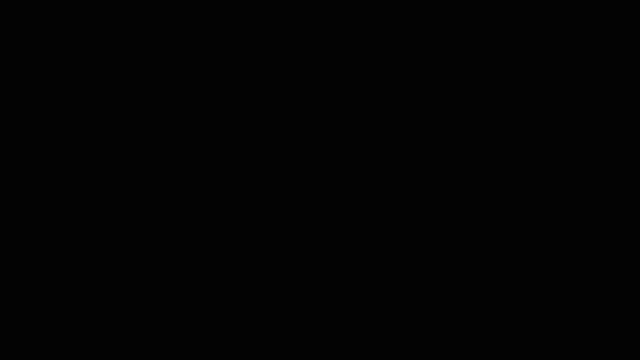 Now let's talk about adding fractions with different denominators. I won't spend too much time talking about this topic, but for those of you who want more information on adding and subtracting fractions, multiplying and dividing fractions or even converting a decimal back into a fraction, check out the links in the description section. 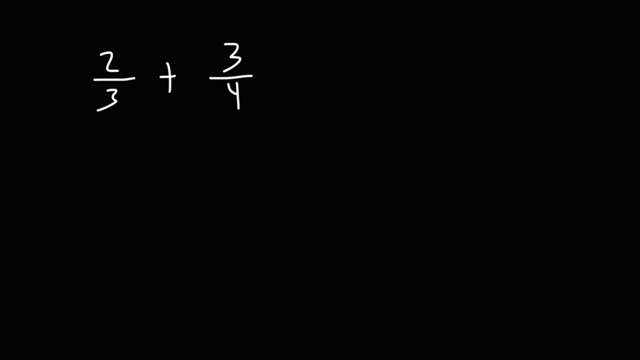 below I'll be posting more video content. I'll be posting more video content there. Also, you can visit my website, wwwvideo-tutornet. On that website you'll find the playlists that I have on math, algebra, trig, pre-calc. 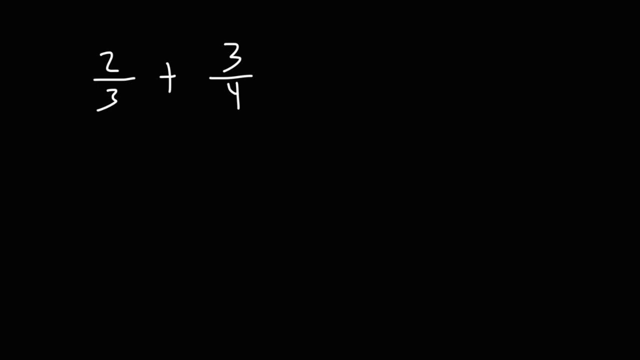 calc, chemistry, physics and other topics that you might be taking, like statistics and trigonometry, So feel free to take a look at that website and the links in the description section below. Now let's talk about adding fractions with unlike denominators. 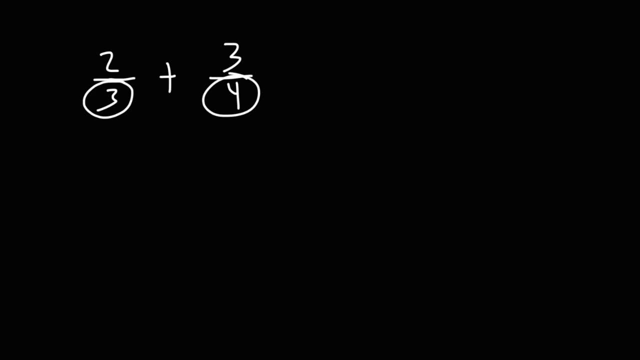 How can I add a fraction? Let's take a look at my website. How can we add these two fractions? Well, we need to get a common denominator To do that. multiply the second fraction by the other denominator, 3.. And if you multiply the denominator by 3, you need to multiply the numerator by 3 as well. 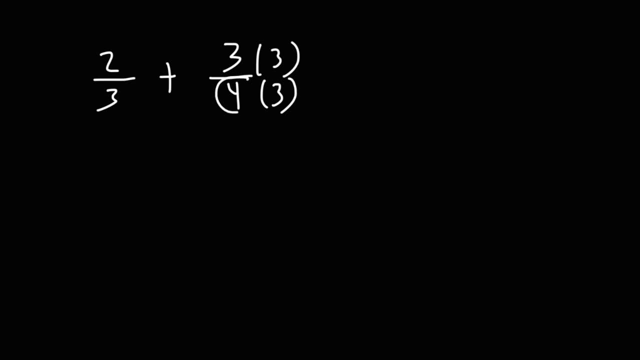 Now for 2 over 3, we're going to multiply that fraction by the other denominator, that is, by 4 over 4.. So this will help us to get the same denominator. at the same time, the value of the fraction is a change. 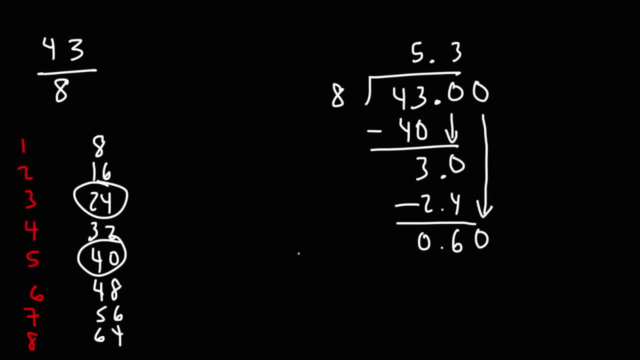 Next we need to add another 0.. 8 goes into 60. seven times 8 times 7 is 56. So the difference between 60 and 56 is 4.. Add another 0.. 8 goes into 40, five times. 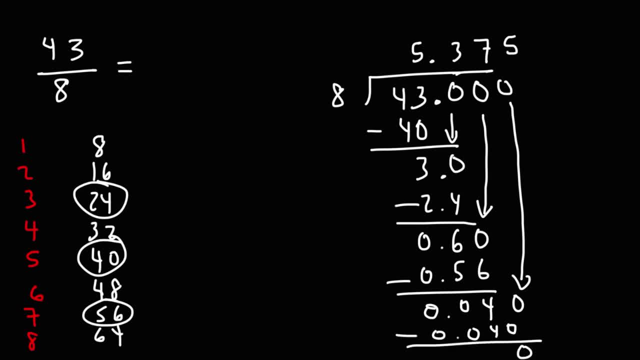 And this gives us a remainder of 0.. So 43 divided by 8 is 5.375.. So that's how you can divide fractions if the denominator doesn't go evenly into the numerator, And that's also how you can convert a fraction. 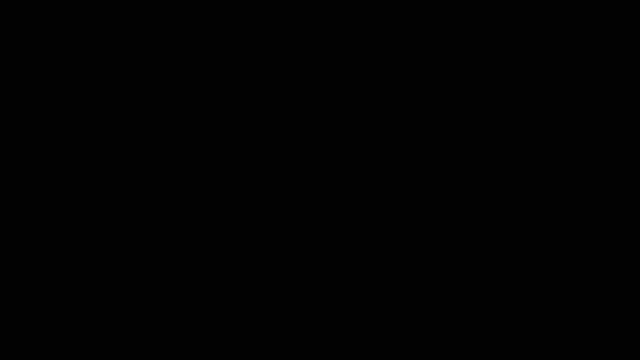 into a decimal. Now let's talk about adding fractions with different denominators. I won't spend too much time talking about this topic, but for those of you who want more information on adding and subtracting fractions, multiplying and dividing fractions, or even converting a decimal back into a fraction, 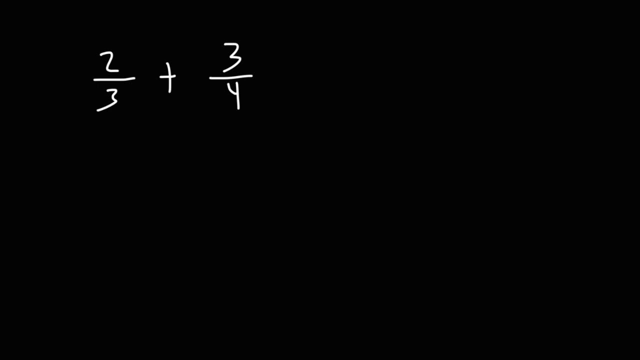 check out the links in the description section below. I'll be posting more video content there. You could also visit my website, wwwvideo-2.0. video-tutornet. On that website you'll find the playlists that I have on math, algebra, trig, precalc, calc. 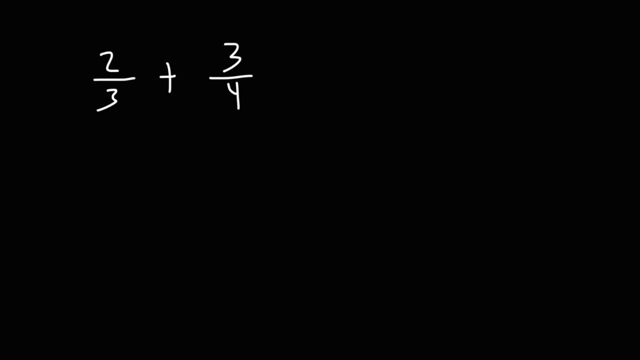 chemistry, physics and other topics that you might be taking, like statistics and trigonometry, So feel free to take a look at that website and the links in the description section below. Now let's talk about adding fractions with unlike denominators. 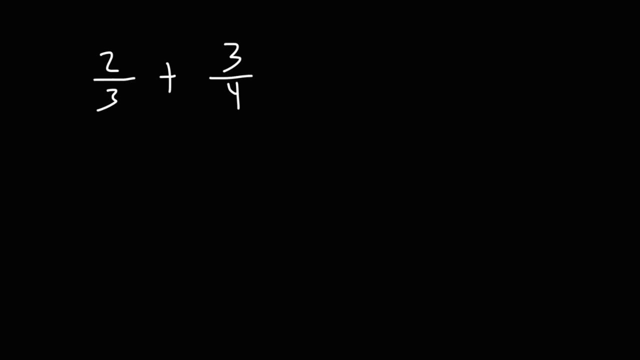 How can we add these two fractions? Well, we need to get a common denominator To do that. multiply the second fraction by the other denominator, 3, and if you multiply the denominator by 3,, you need to multiply the numerator by 3 as well. 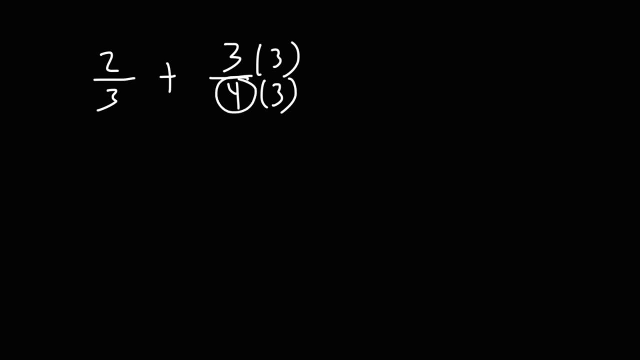 Now for 2 over 3, we're going to multiply that fraction by the other denominator, that is, by 4 over 4.. So this will help us to get the same denominator. at the same time, the value of the fraction is a change. 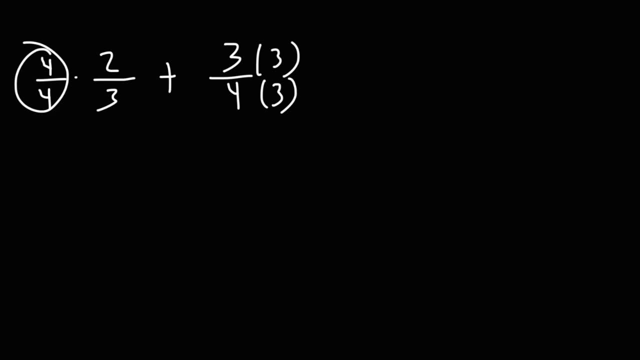 4 over 4 is 1.. If you multiply 2 thirds by 1, it remains 2 thirds. 3 over 3 is 1.. Multiplying 3 fourths by 1, the value of the fraction stays 3 fourths. 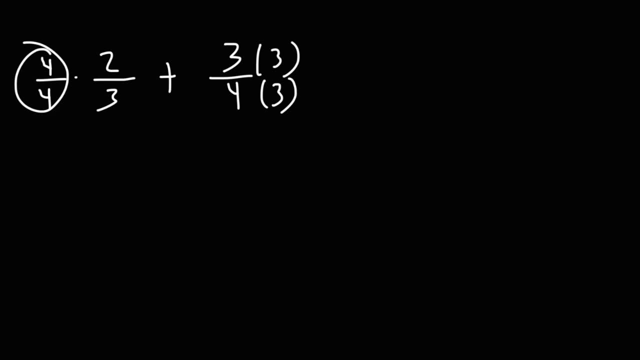 4 over 4 is 1.. If you multiply 2 thirds by 1, it remains 2 thirds. 3 over 3 is 1.. Multiplying 3 fourths by 1, the value of the fraction stays 3 fourths. 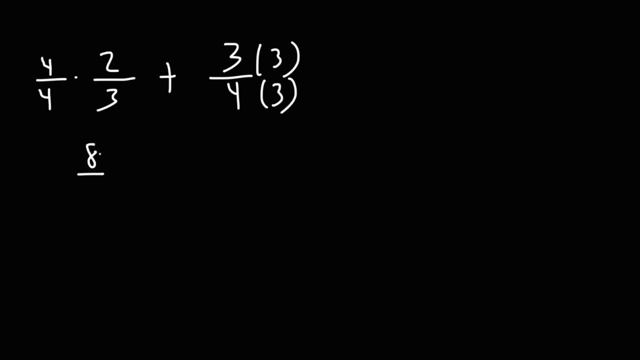 4 times 2 is 8. And then 4 times 3 is 12.. 3 times 3 is 9. And 4 times 3 is 12.. So notice that 8 over 12. And 2 over 3, they have the same value. 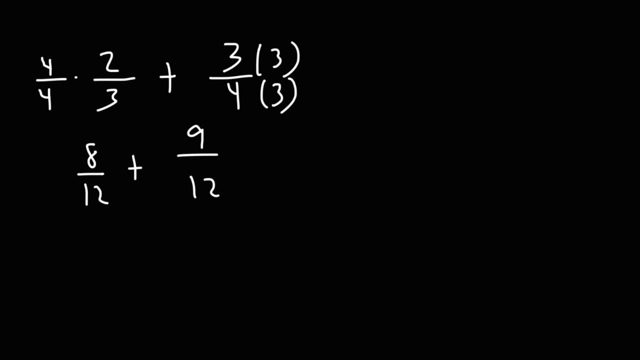 8 over 12 reduces to 2 over 3.. But now these two fractions have the same denominator. As a result, we can add the numerators of the two fractions: 8 plus 9 is 17.. So the answer is 17 over 12.. 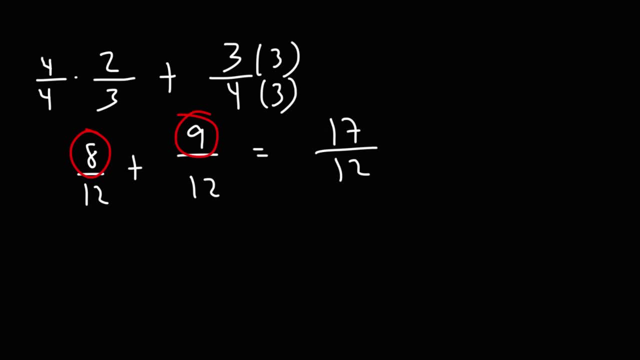 That's the answer as an improper fraction. To convert this into a mixed number, you can break down 17 into 12 and 5.. 12 plus 5 is 17.. 12 divided by 12 is 1.. So you get 1 plus 5 over 12.. 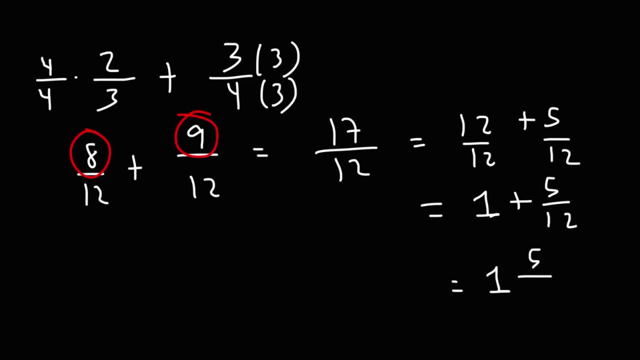 You can write that as 1 and 5 twelves, So that's a simple way of how you can convert an improper fraction into a mixed number. An improper fraction is a fraction where the numerator exceeds the value of the denominator. Now let's talk about subtracting fractions. 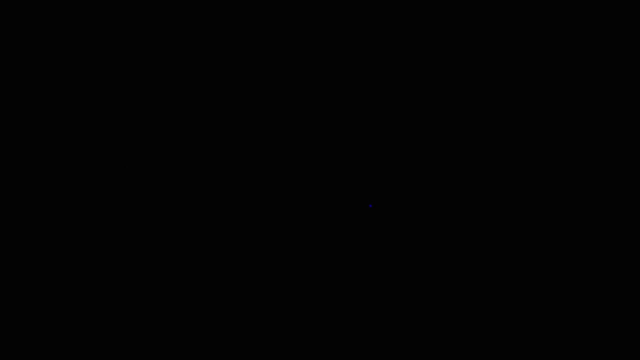 So let's say that the numerator exceeds the value of the denominator. Now let's talk about subtracting fractions. So let's say: Let's say we have 4 over 5 and we wish to subtract it by 1 over 7.. 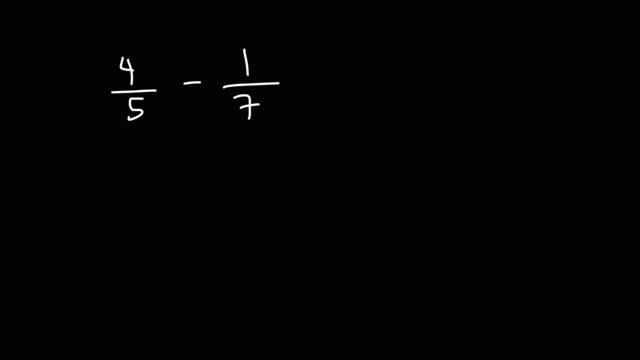 What do we need to do here? Just like before when we were adding fractions, we need to get common denominators. So we're going to multiply the first fraction by the other denominator, that is, by 7 over 7, and we're going to multiply the second fraction by the first denominator, that is. 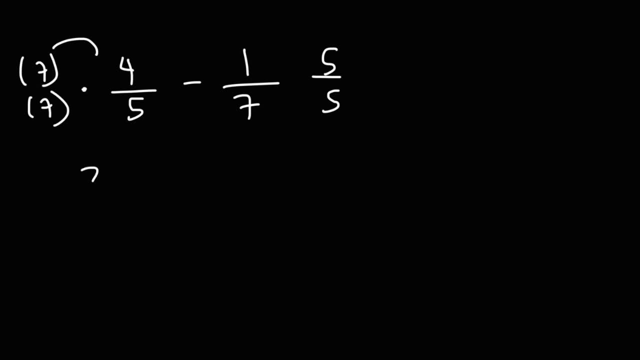 by 5 over 5.. 7 times 4 is 28,, and then 7 times 5 is 35.. One times 5 is 5, and the bottom is going to be 35 as well. So, now that we have the same denominator, we can now subtract the numerators of the. 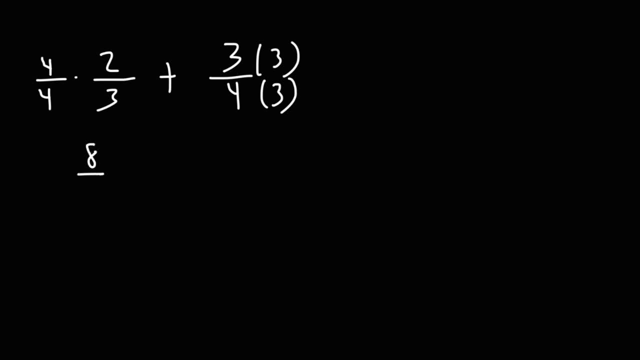 4 times 8,. I mean 4 times 2 is 8, and then 4 times 3 is 12.. 3 times 3 is 9, and 4 times 3 is 12.. So notice that 8 over 12 and 2 over 3,. 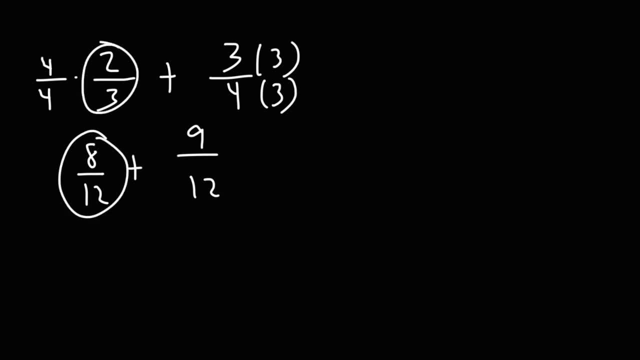 they have the same value. 8 over 12 reduces to 2 over 3.. But now these two fractions have the same denominator. As a result, we can add the numerators of the two fractions. 8 plus 9 is 17,. 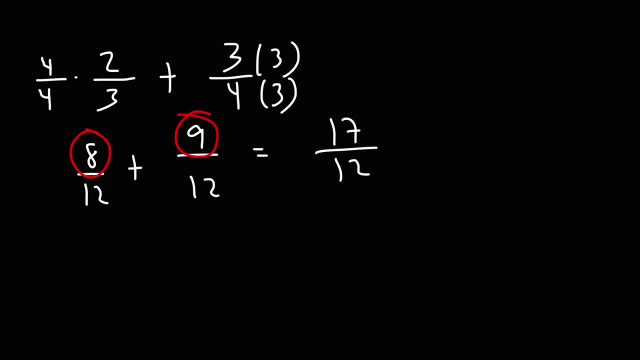 so the answer is 17 over 12.. That's the answer as an improper fraction. To convert this into a mixed number, you can break down 17 into 12 and 5.. 12 plus 5 is 17.. 12 divided by 12 is 1.. 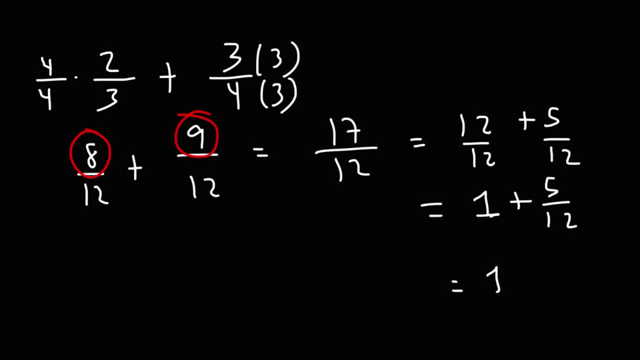 So you get 1 plus 5 over 12, and you can write that as 1 and 5 twelfths. So that's a simple way of how you can convert an improper fraction into a mixed number. An improper fraction is a fraction where 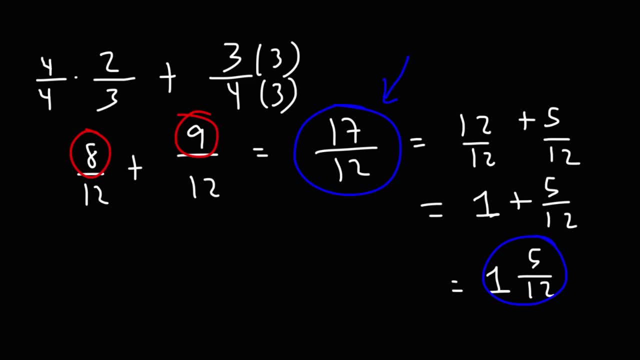 the numerator exceeds the value of the denominator. Now let's talk about subtracting fractions. So let's say we have 4 over 5, and we wish to subtract it by 1 over 7.. What do we need to do here? 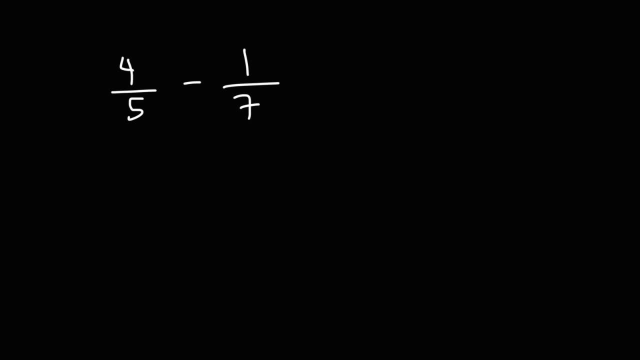 Just like before when we were adding fractions, we need to get common denominators. So we're going to multiply the first fraction by the other denominator, That is, by 7 over 7.. And we're going to multiply the second fraction by the first denominator. 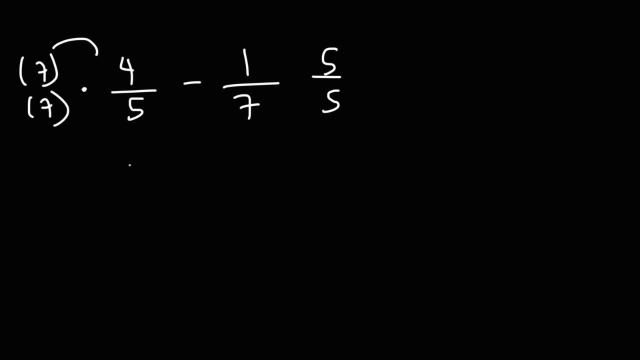 That is, by 5 over 5.. 7 times 4 is 28,, and then 7 times 5 is 35.. 1 times 5 is 5, and the bottom is going to be 35 as well. So now that we have the same denominator, 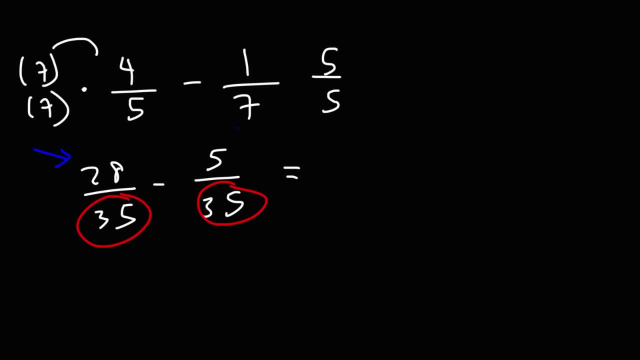 we can now subtract the numerators of the two fractions, So 28 minus 5 is 23.. So the final answer is 23 over 35.. Now the numerator is less than the denominator, so this is not an improper fraction. So thus this is our final answer. 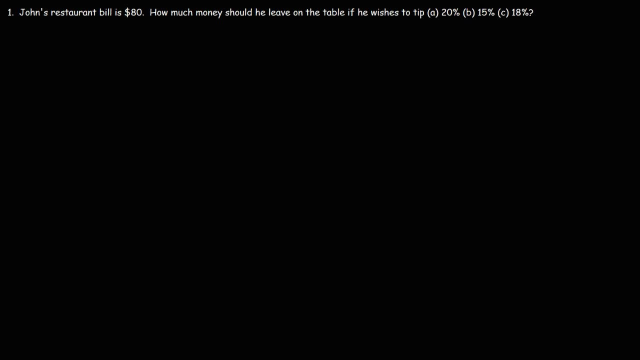 Now the last concept that we're going to cover in this video is percentages. Let's look at this problem. John's restaurant bill is $80.. How much money should he leave on the table if he wishes to tip 20%? Now, sometimes, if you're at a restaurant, 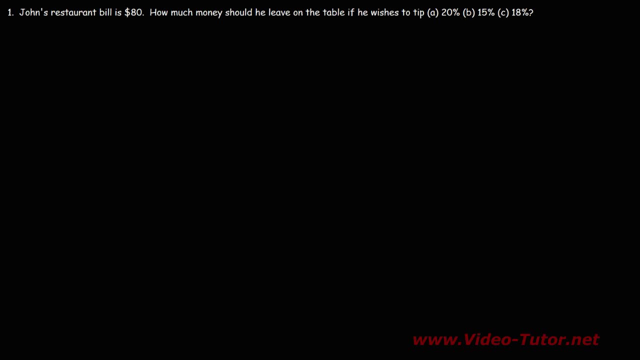 and you want to decide how much you want to tip, it's good to do some mental math. You don't always have a calculator with you Now, granted, you could use your cell phone, but this is a good instance where it's good to know mental math. 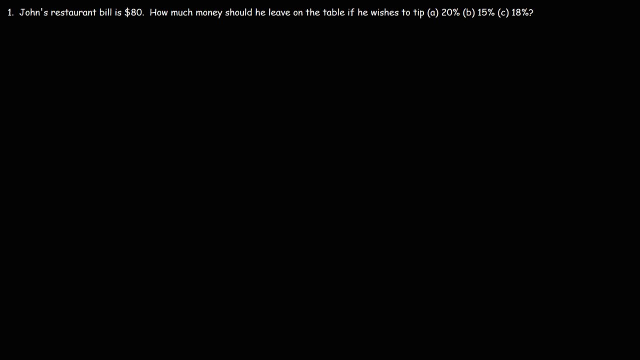 in order to get like a ballpark figure, if you want to tip 15% or 20%, which is what is customarily given for tips. Now, in this problem, we're not looking for the total price, that is the $80 bill plus a tip. 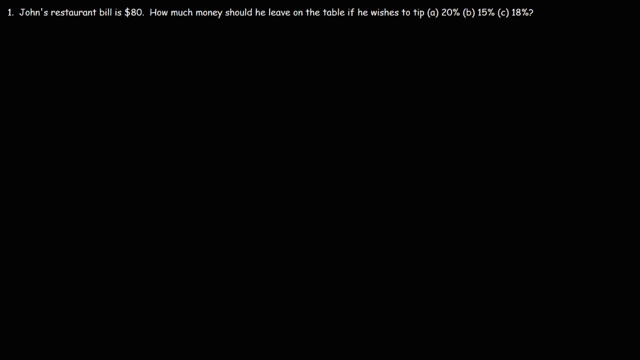 We just want to know the value of the tip that he should leave on the table. So in Part A we want to find out what is 20% of 80.. So let's talk about how to do this mentally First. what is 10% of 80?? 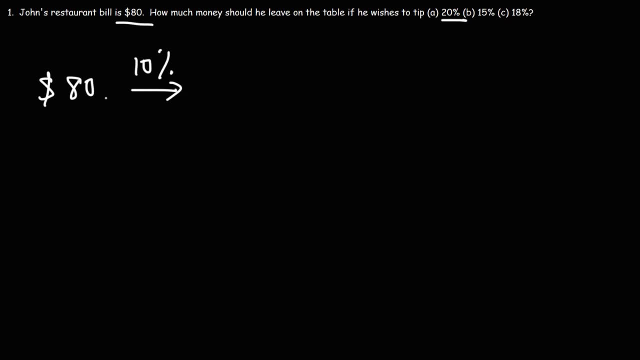 To calculate 10% of anything, move the decimal point one unit to the left. So 10% of 80 is simply 8.. Now if 10% is $8,, how much is 20%? 20% is twice the value of 10%. 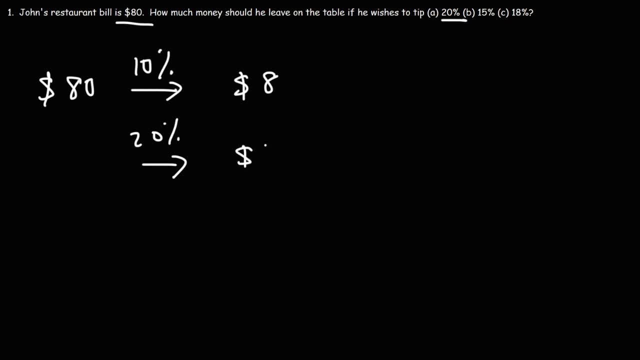 So it's going to be twice the value of $8 or $16.. So that's how much money he should leave on a table. The other way to calculate the value of 20%: take $80 and multiply it by 20% as a decimal. 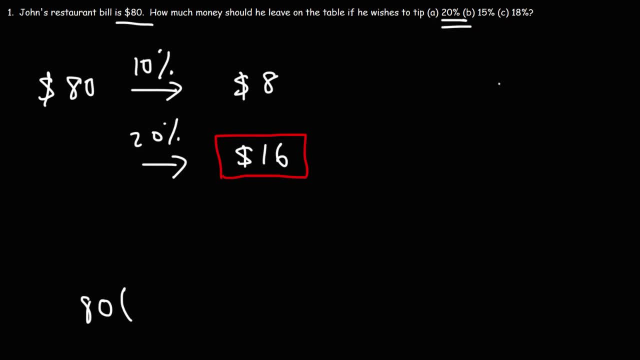 To convert a percentage into a decimal, divide it by 100, or you could move the decimal point two units to the left. So 20% as a decimal is .20.. So if you were to type in 80 times .20,. 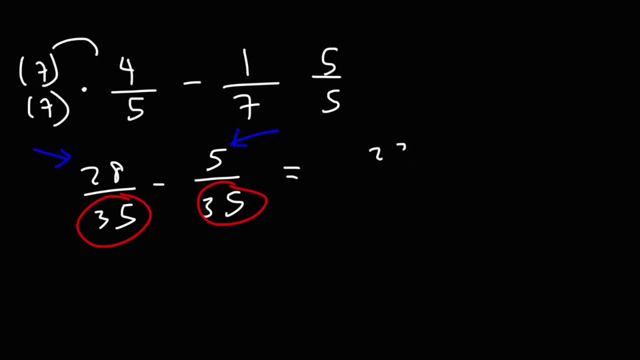 two fractions. So 28 minus 5 is 23.. So the final answer is 23 over 35.. Now, the numerator is less than the denominator, so this is not an improper fraction. So thus this is our final answer. Now, the last concept that we're going to cover in this video is percentages. 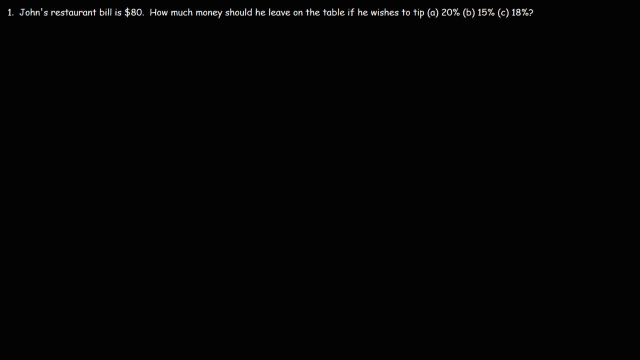 Let's look at this problem. John's restaurant bill is $80.. How much money should he leave on the table if he wishes to tip 20%? Now, sometimes, if you're at a restaurant and you want to decide how much you want to tip, 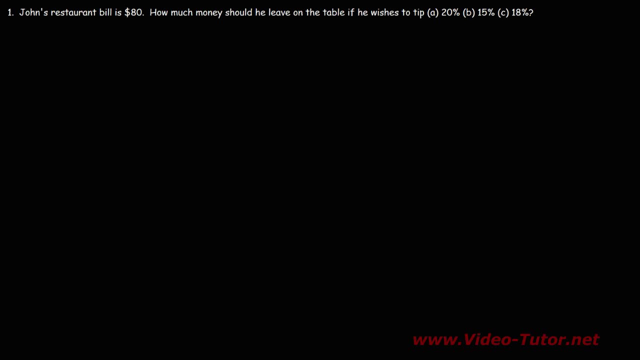 it's good to do some mental math. You don't always have a calculator with you. Now, granted, you could use your cell phone. This is a good instance where it's good to know mental math in order to get like a ballpark figure if you want to tip 15% or 20%, which is what is customarily given for tips. 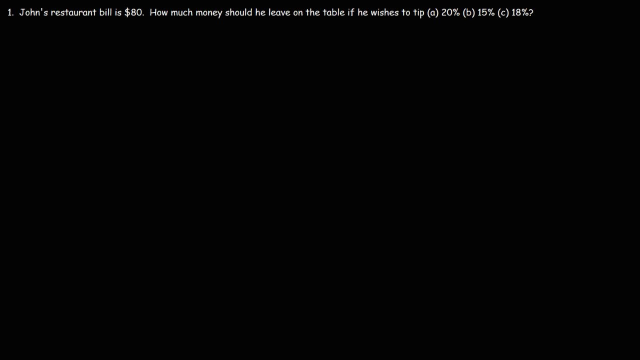 Now, in this problem we're not looking for the total price, that is, the $80 bill plus a tip. We just want to know the value of the tip that he should leave on the table. So in part A we want to find out what is 20% of 80.. 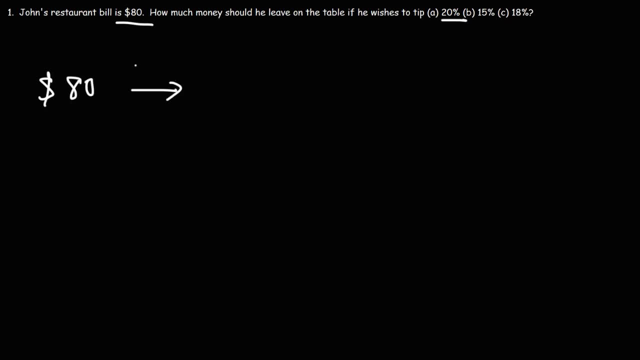 So let's talk about how to do this mentally. First, we want to know the value of the tip that he should leave on the table. First, what is 10% of 80?? To calculate 10% of anything, move the decimal point one unit to the left. 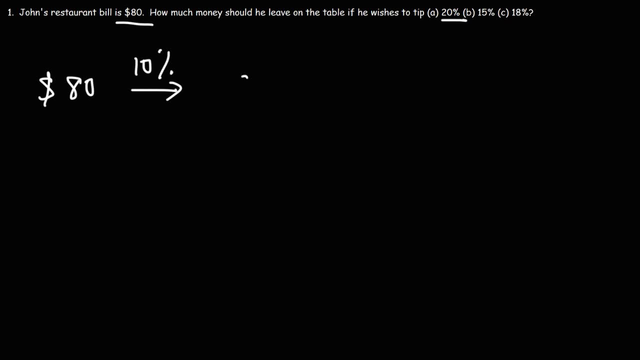 So 10% of 80 is simply 8.. Now if 10% is $8,, how much is 20%? 20% is twice the value of 10%, So it's going to be twice the value of $8 or $16.. 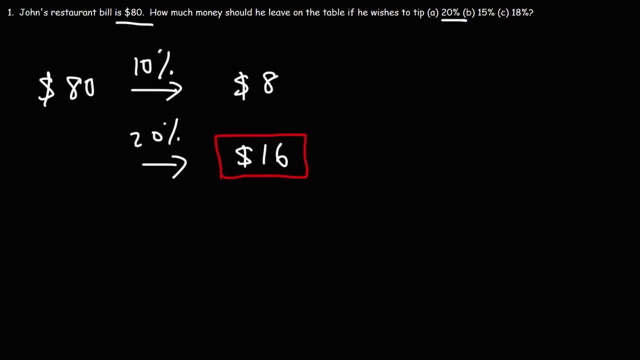 So that's how much money he should leave on a table. To calculate the value of 20%, take $80 and multiply it by 20% as a decimal. To convert a percentage into a decimal, divide it by 100, or you could move the decimal point. 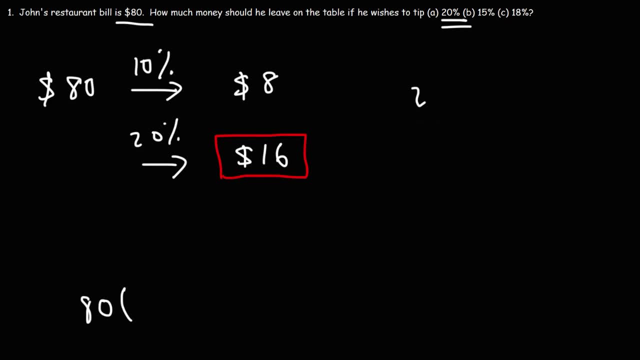 two units to the left. So 20% as a decimal is .20.. So if you were to type in 80 times .20,, you would also get 16.. Now let's move on to Part B. What is 15% of $80?? 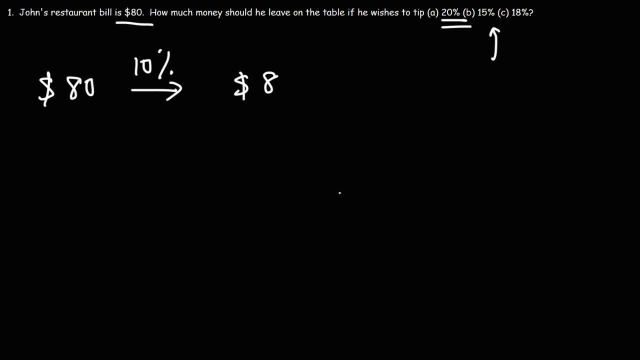 So if he wants to give a 15% tip, how much money should he leave on the table? Well, we know that 10% is $8.. What is 5%? 5% is half of 10%, So half of 8 is 4.. 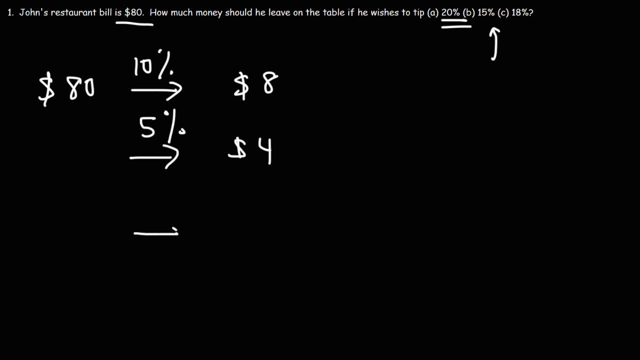 Thus 5% of 80 is $4.. Now to get 15% we simply need to add 10% and 5%. So 8 plus 4 is $12.. So if he wishes to give a 15% tip, he needs to leave $12 on the table. 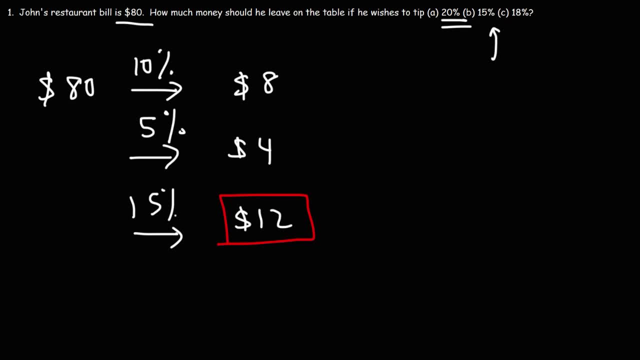 Now what about 18%? Let's see how we can calculate that. If 10% is $8,, what is 1% of 80?? To calculate 1%, move the decimal two units to the left. 1% is going to be 80 cents. 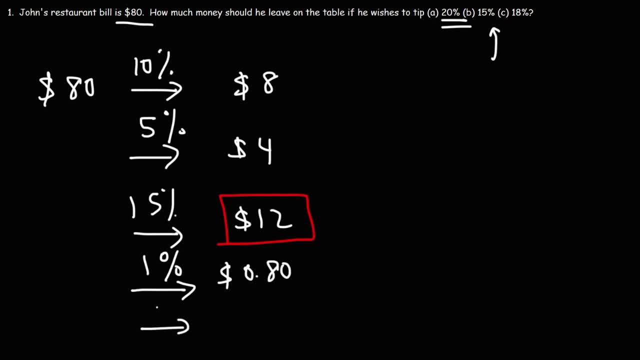 Now let's move on to Part B. Now, if 1% is 80 cents, what's 3%? Well, 3% is 3 times the value of 1%, So it's 3 times 80 cents. We know that 3 times 8 is 24.. 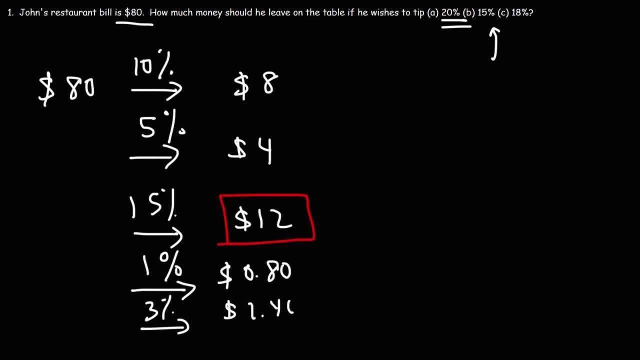 So 3 times 80 cents will be $2.40.. So to get 18%, we simply need to add 15% and 3%. So we need to add 12 and $2.40, which will give us $14.40.. 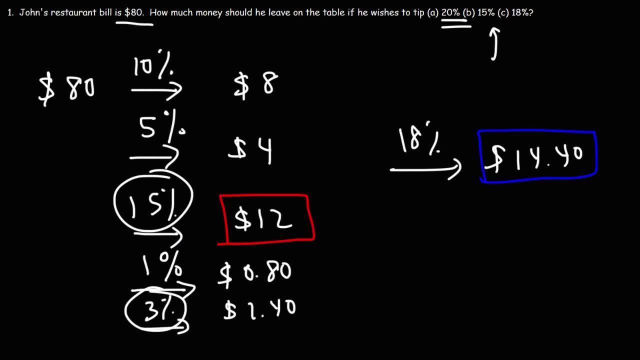 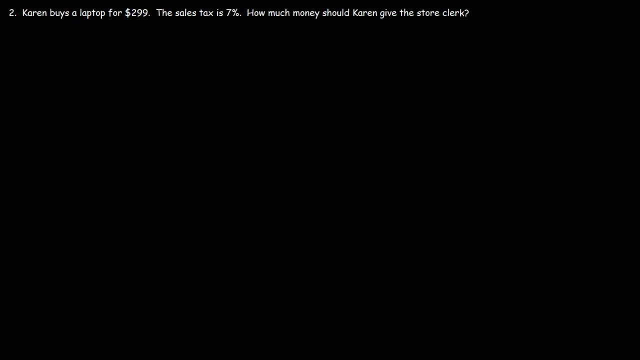 So that will be 18% And 18% tip, That's 18% of $80.. To confirm it, multiply 80 by .18.. 80 times .18 is $14.40.. Now let's work on another percentage-based word problem. 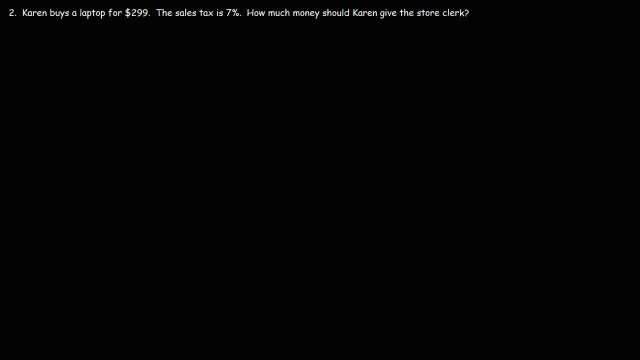 By the way, for those of you who want more word problems on percentages, check out the links in the description section below Number 2.. Karen buys a laptop for $2.50.. Karen buys a laptop for $299.. 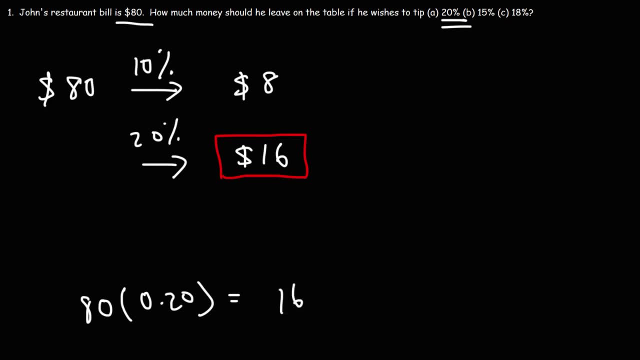 you would also get 16.. Now let's move on to Part B. What is 15% of $80?? So if he wants to give a 15% tip, how much money should he leave on the table? Well, we know that 10% is $8.. 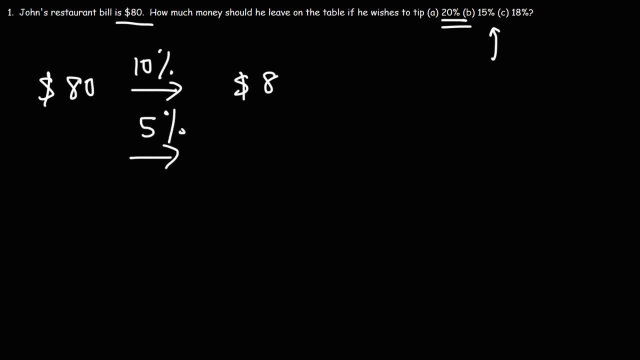 What is 5%? 5% is half of 10%, So half of 8 is 4.. Thus, 5% of 80 is $4.. Now to get 15%, we simply need to add 10% and 5%. 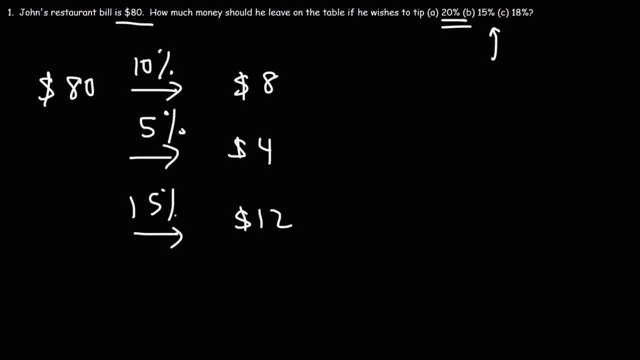 So 8 plus 4 is $12.. So if he wishes to give a 15% tip, he needs to leave $12 on the table. Now what about 18%? Let's see how we can calculate that If 10% is $8,. 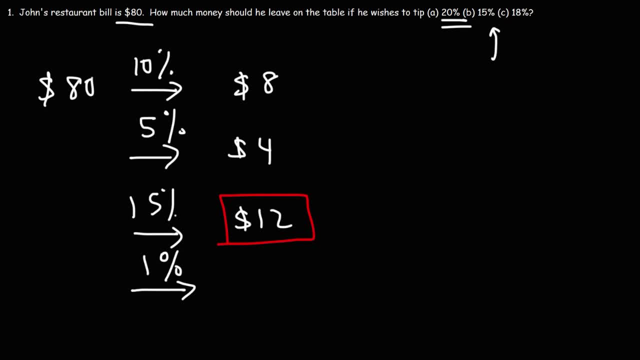 what is 1% of 80?? To calculate 1%, move the decimal two units to the left. 1% is going to be $0.80.. Now if 1% is $0.80, what is 3%? 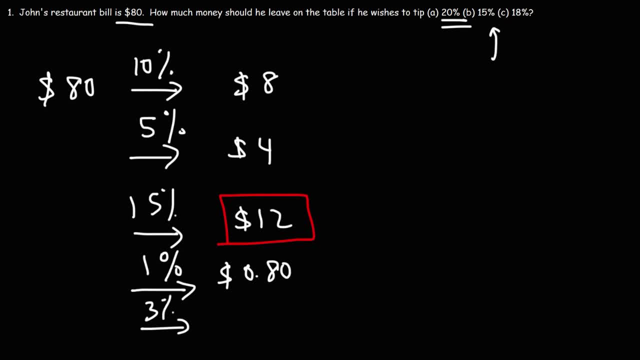 Well, 3% is 3 times the value of 1%, So it's 3 times $0.80.. We know that 3 times 8 is 24.. So 3 times $0.80 will be $2.40.. 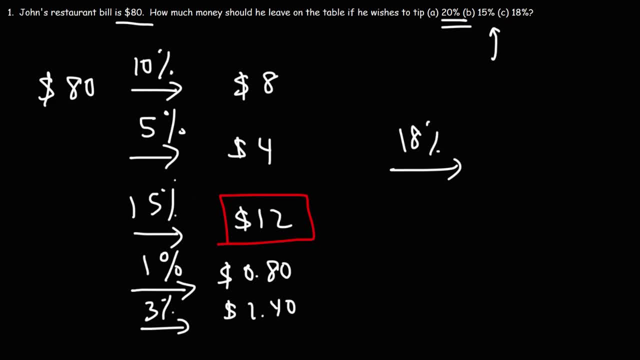 So to get 18%, we simply need to add 15% and 3%. So we need to add 12% and 2% to $2.40, which will give us $14.40.. So that will be an 18% tip. 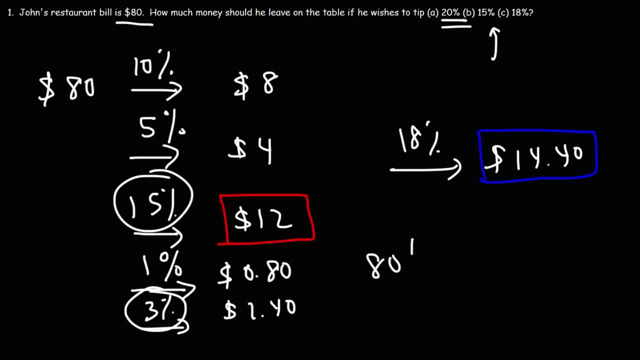 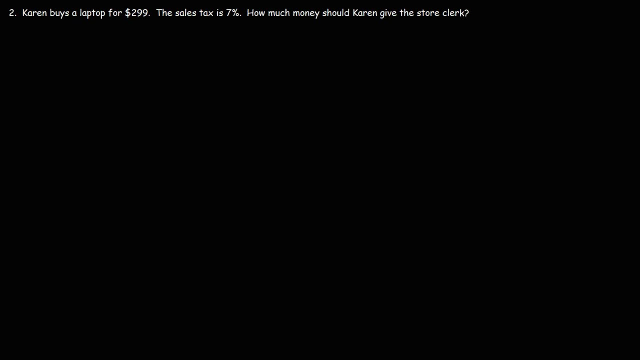 That's 18% of $80.. To confirm it, multiply 80 by 0.18.. 80 times 0.18 is $14.40.. Now let's work on another percentage-based word problem. By the way, for those of you who want more word problems, 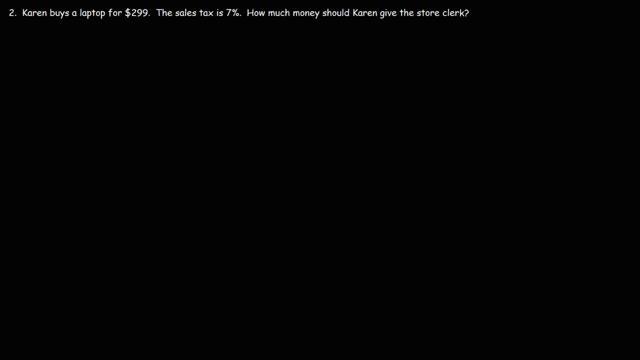 on percentages. check out the links in the description section below Number 2.. Karen buys a laptop for $299.. The sales tax is 7%. How much money should Karen give the store clerk? So in this case it's best to use a calculator for this problem.